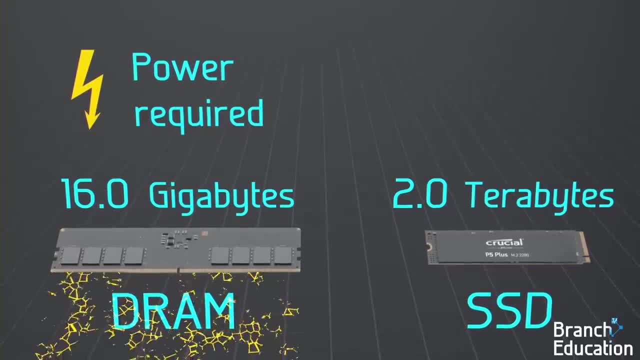 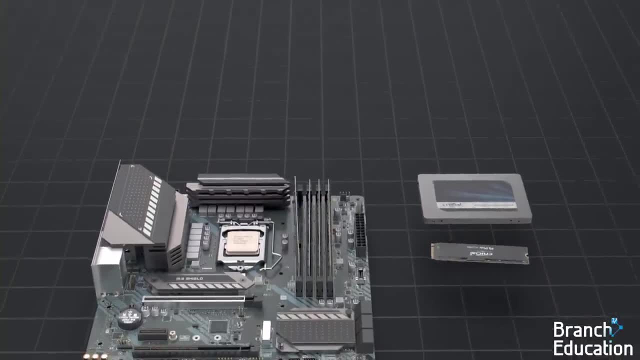 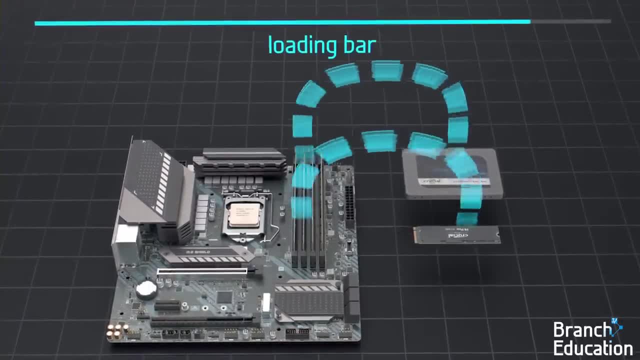 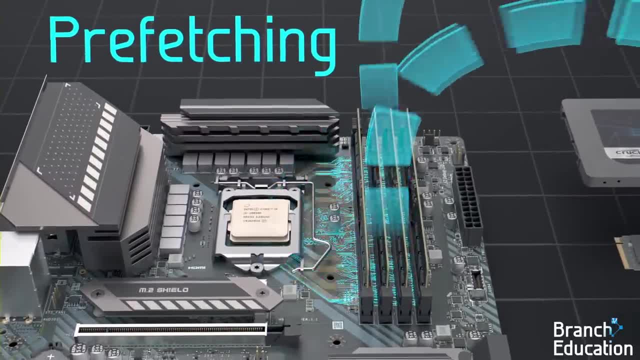 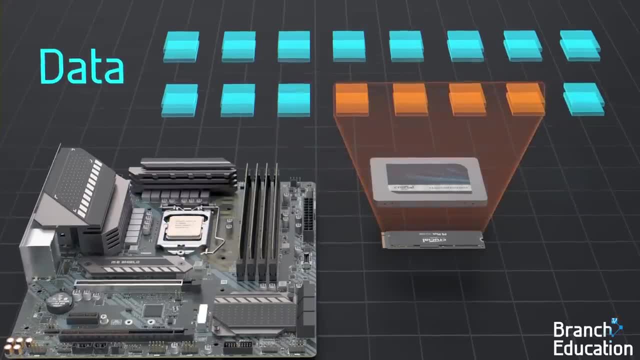 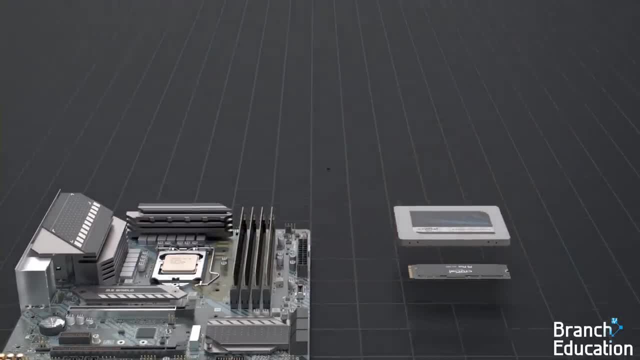 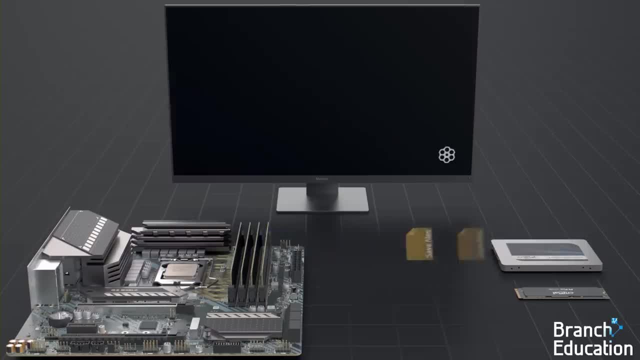 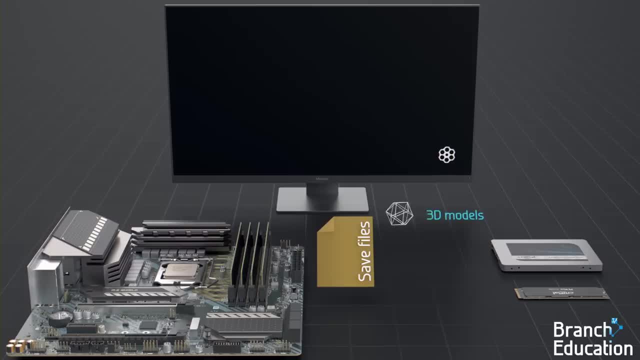 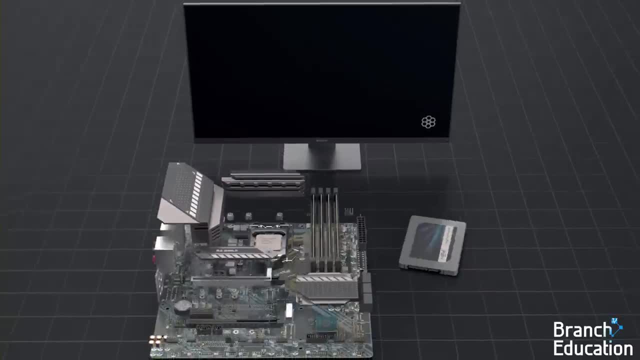 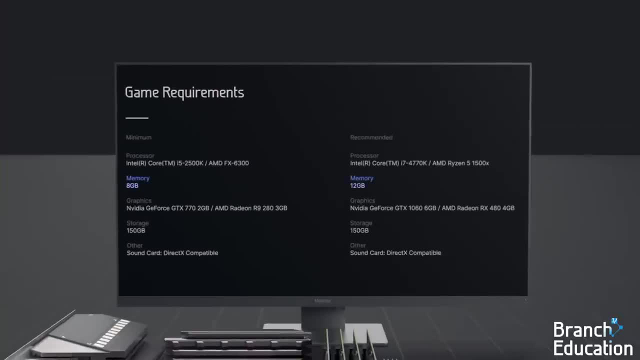 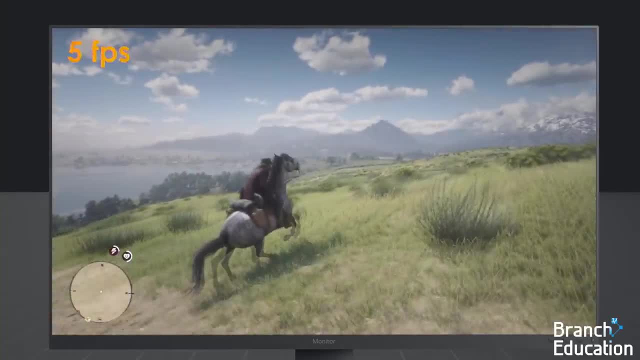 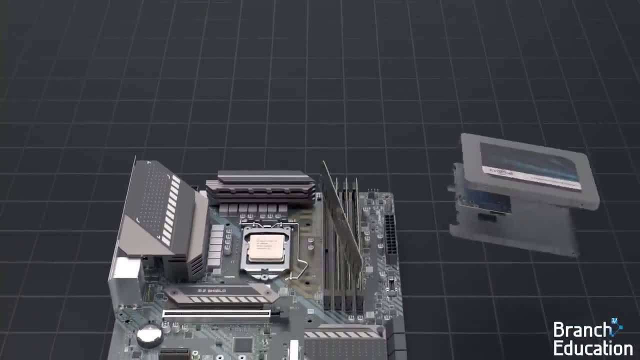 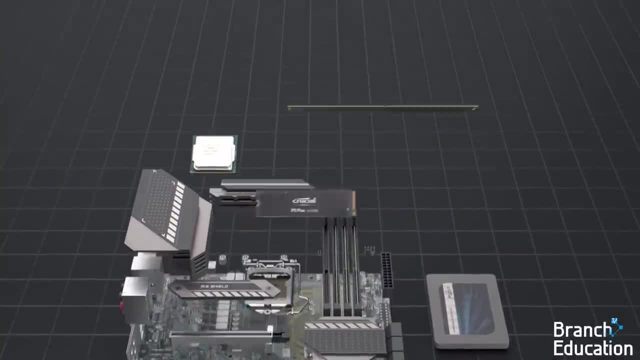 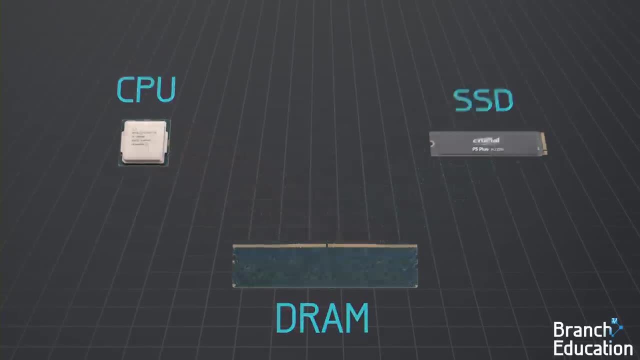 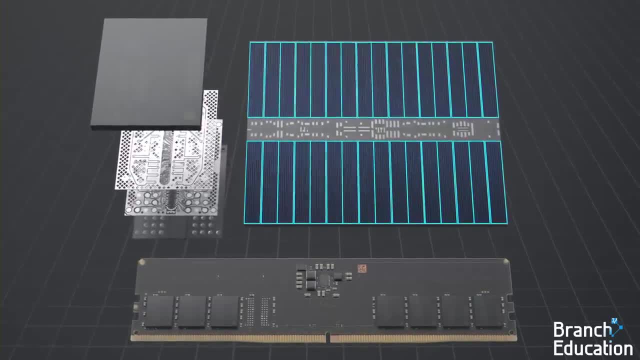 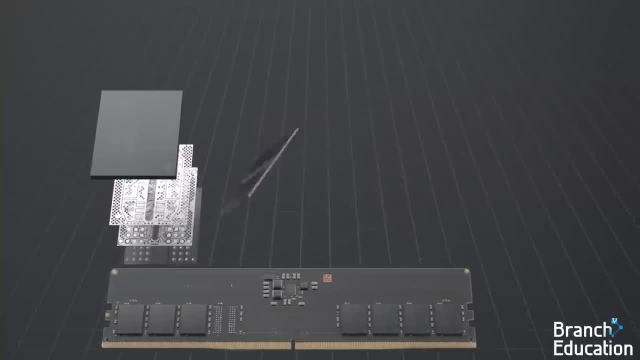 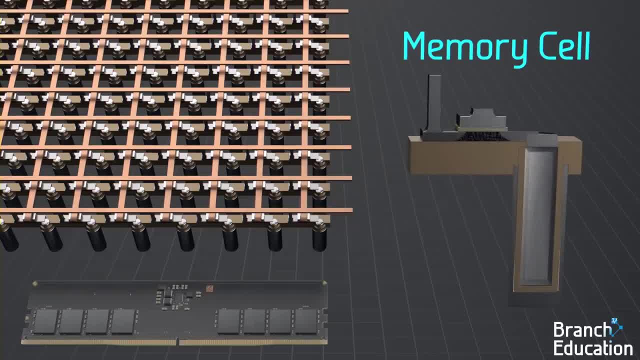 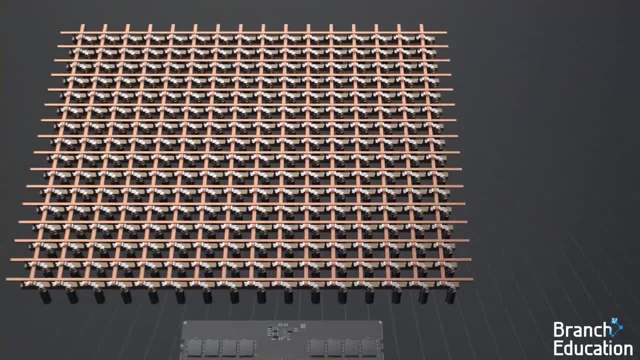 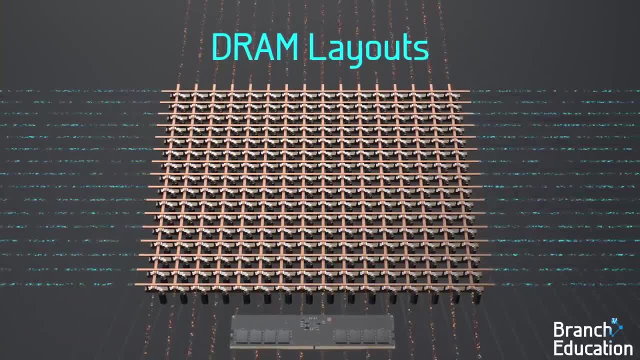 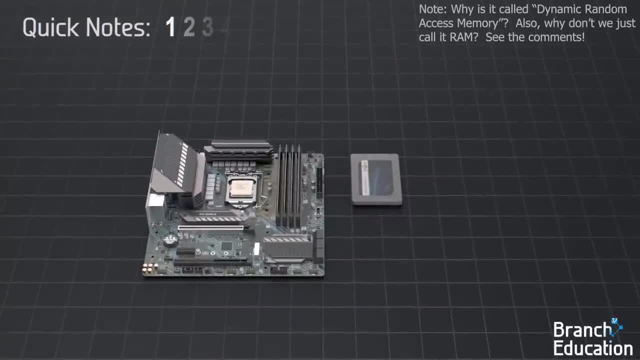 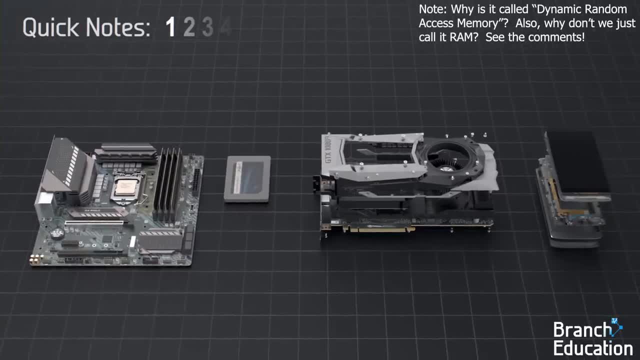 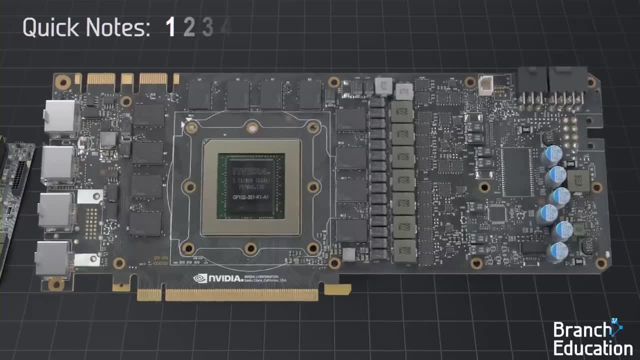 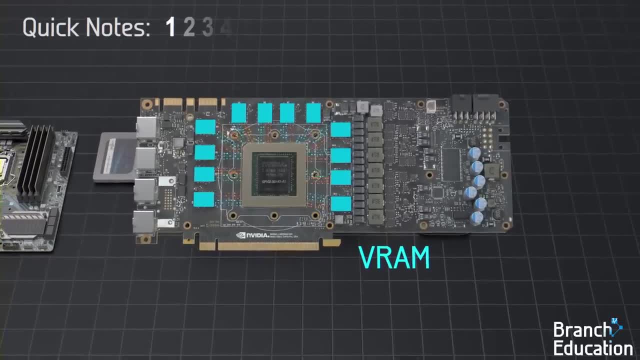 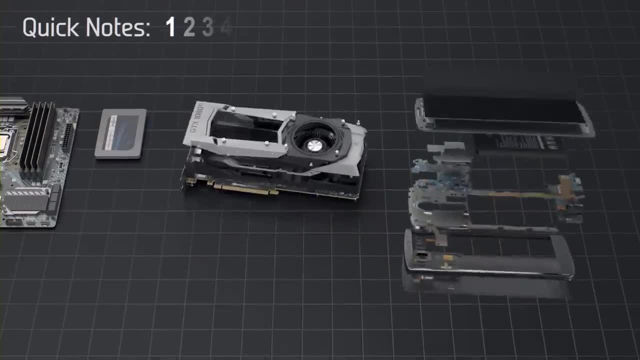 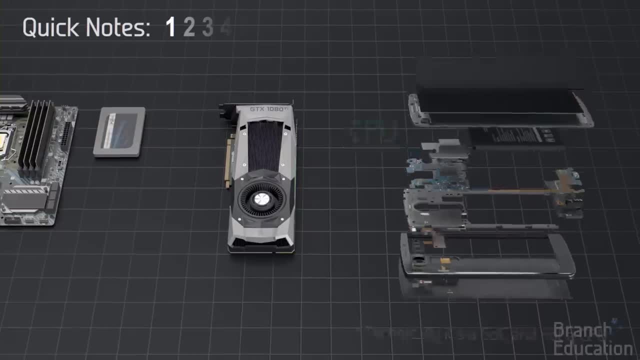 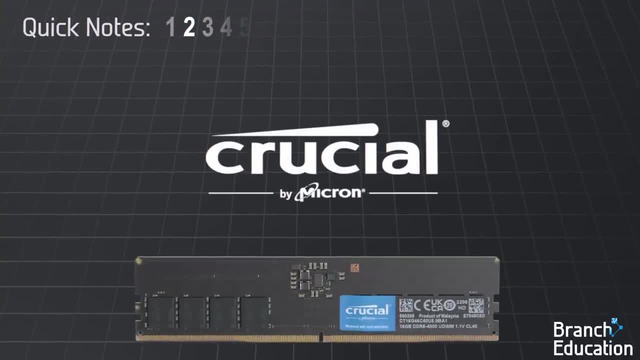 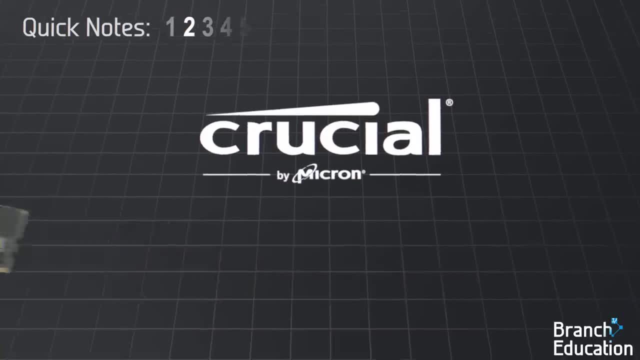 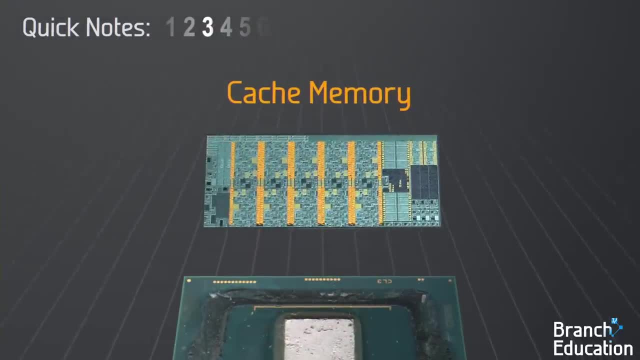 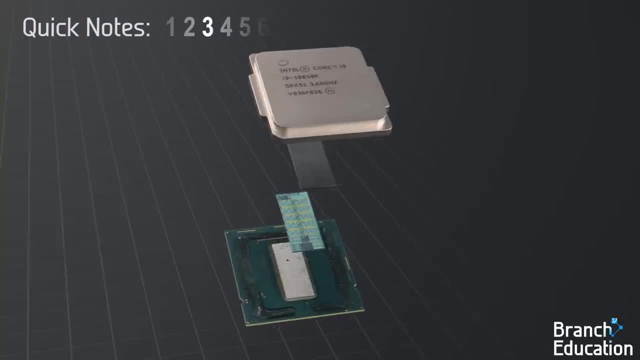 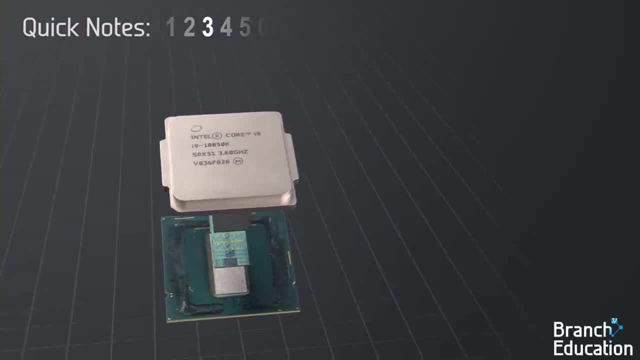 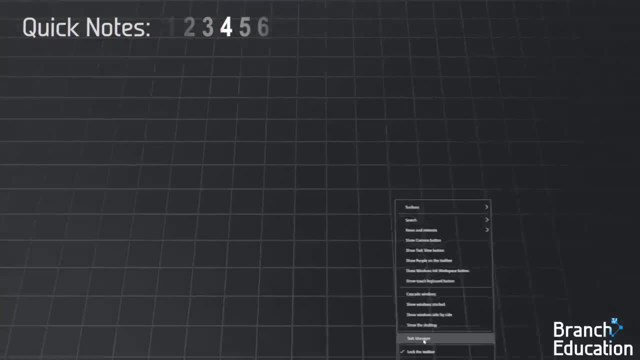 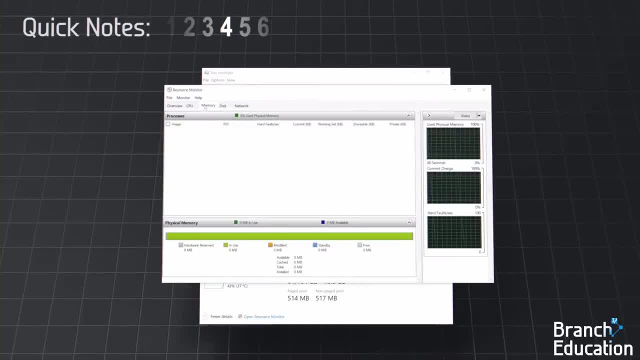 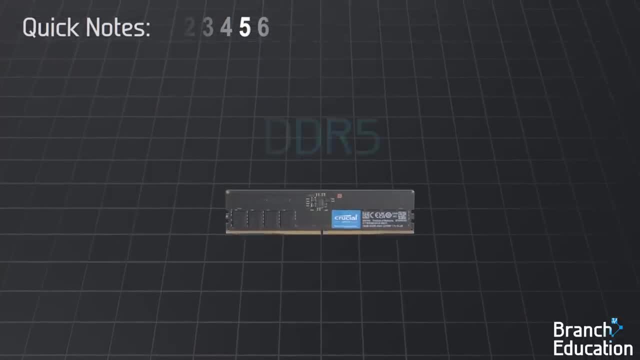 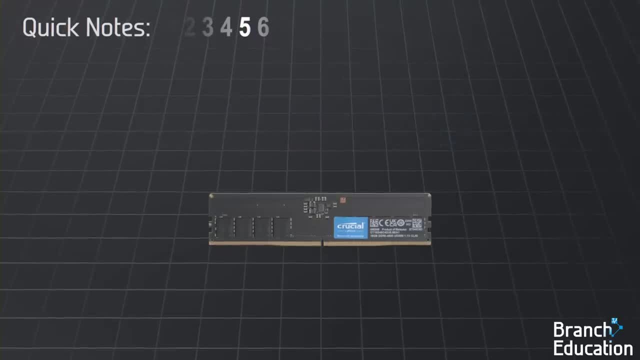 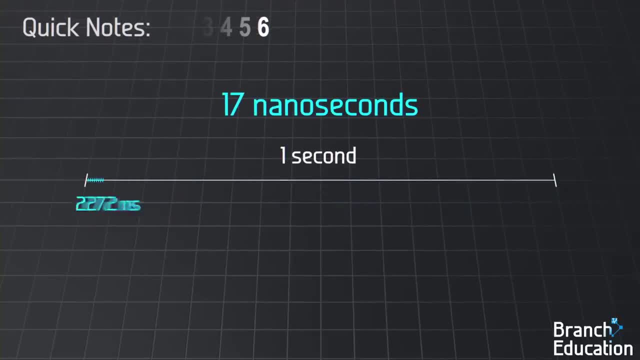 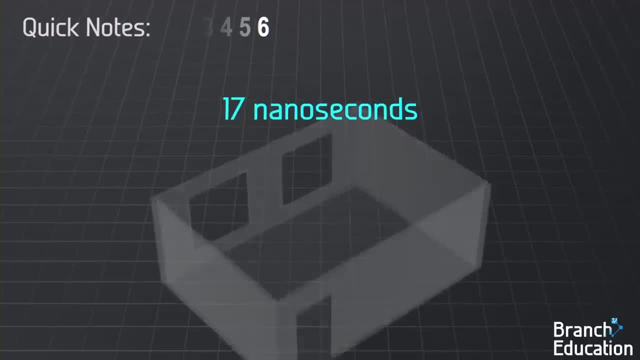 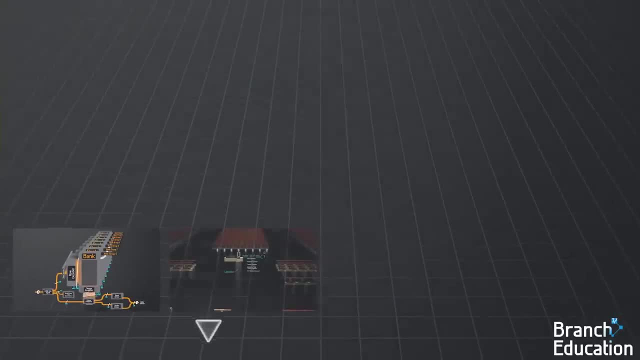 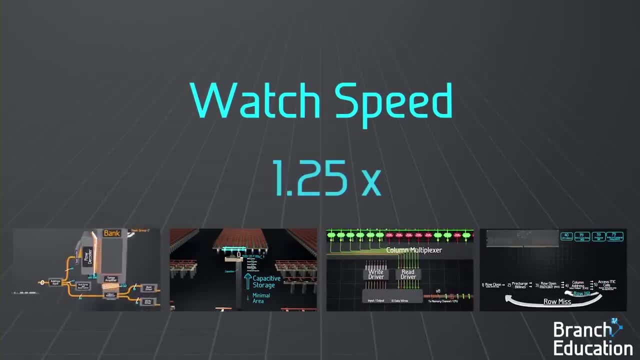 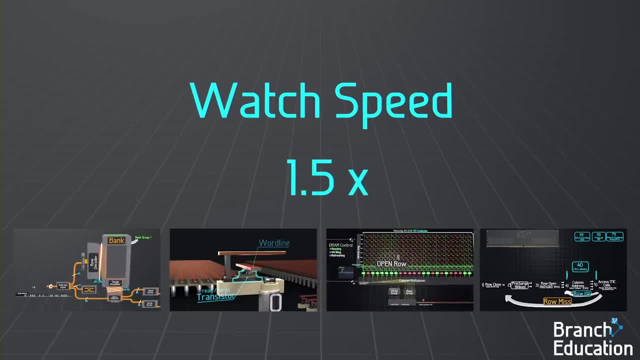 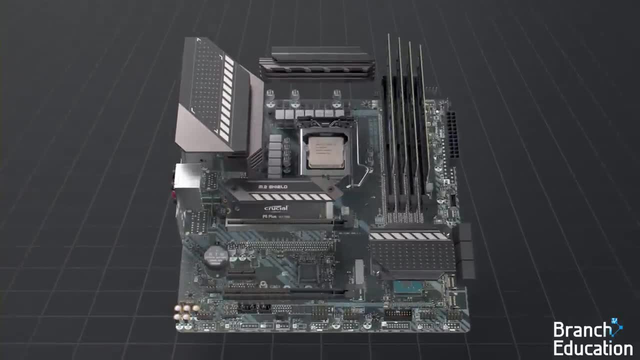 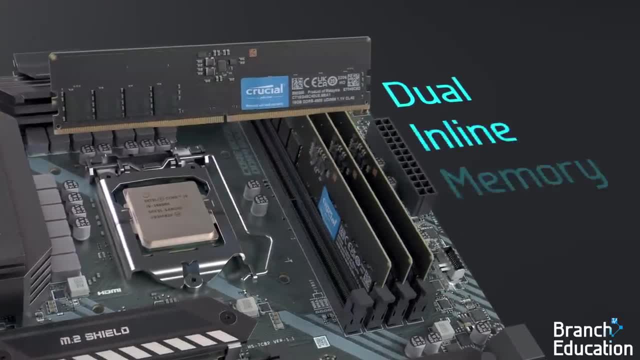 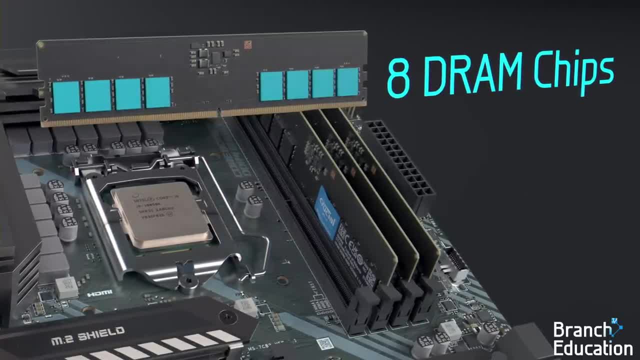 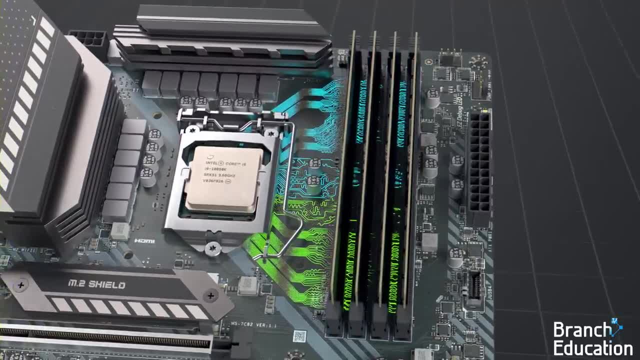 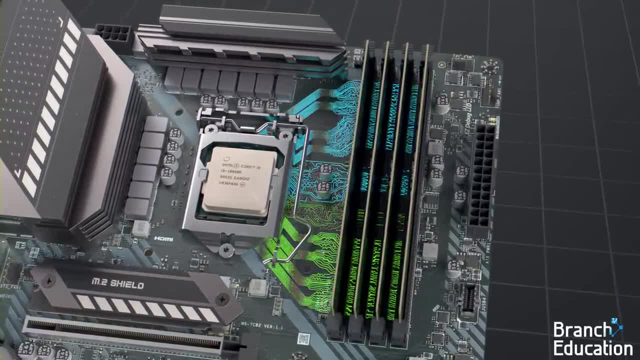 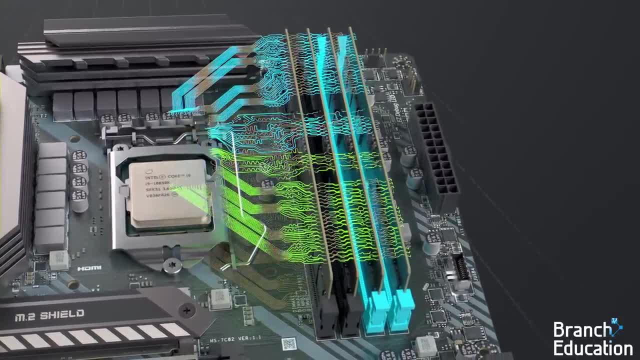 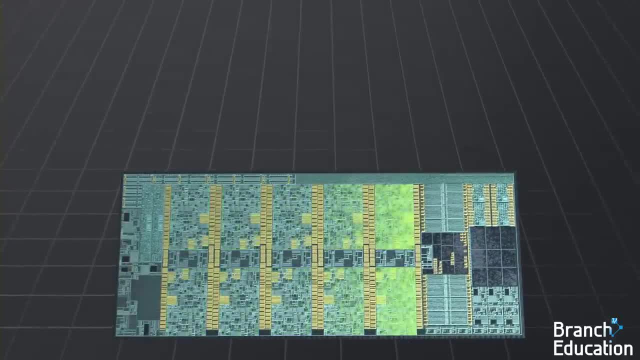 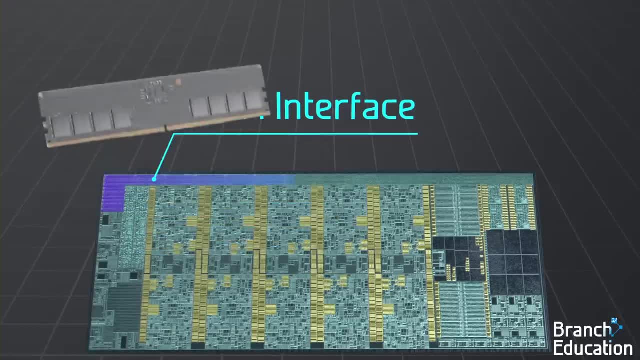 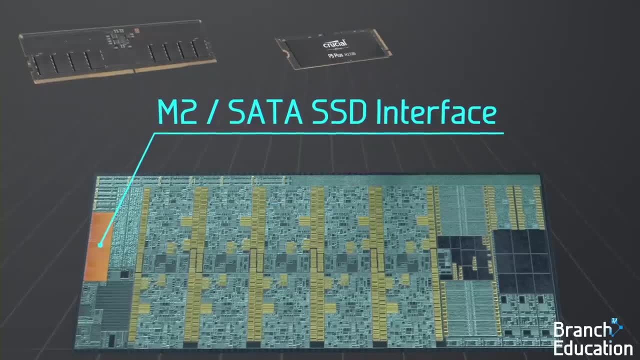 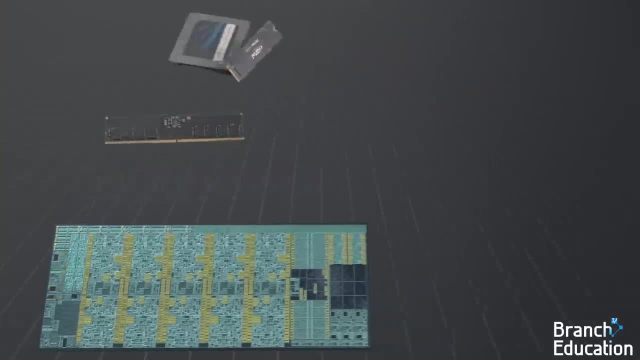 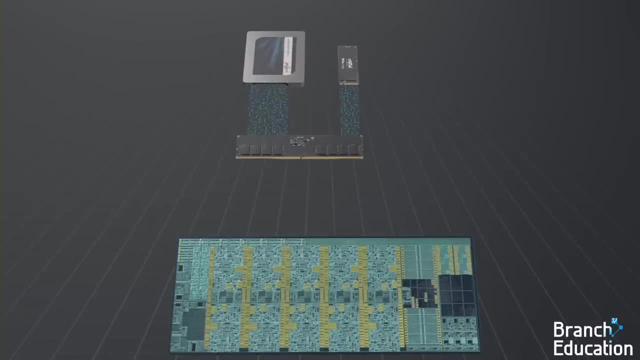 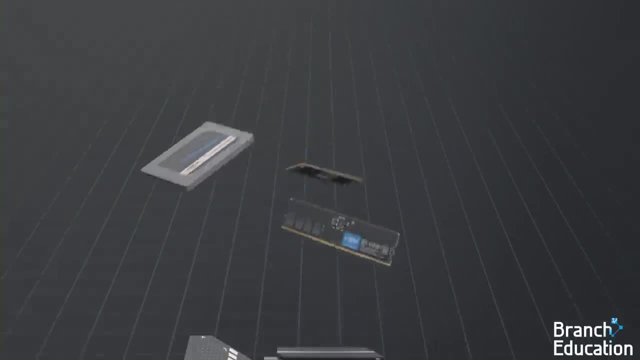 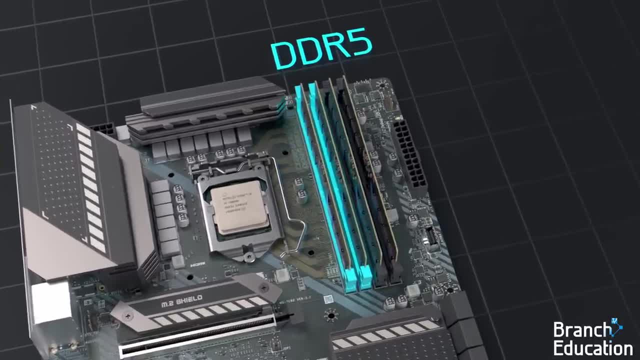 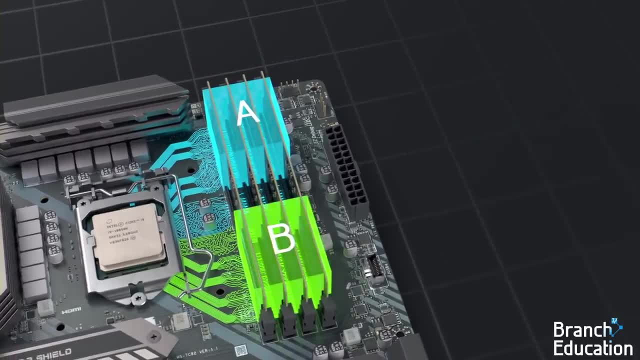 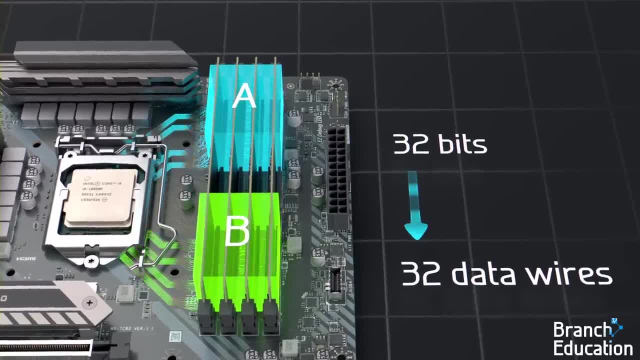 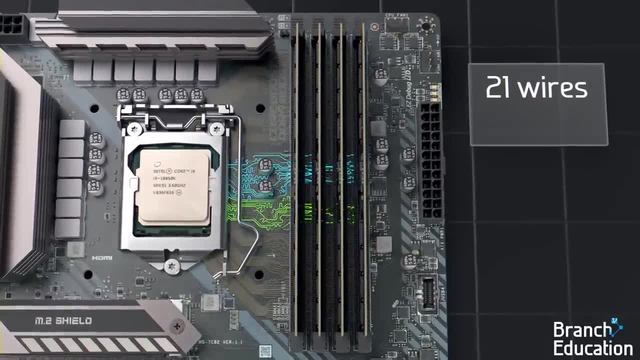 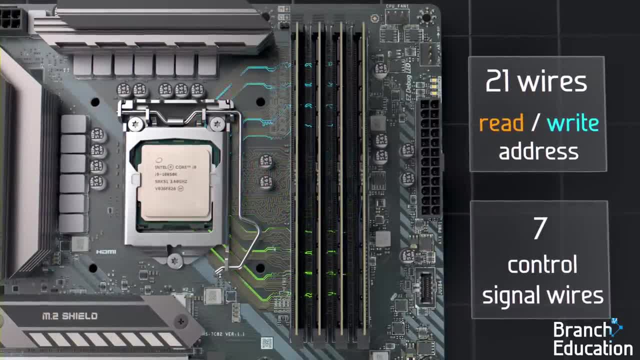 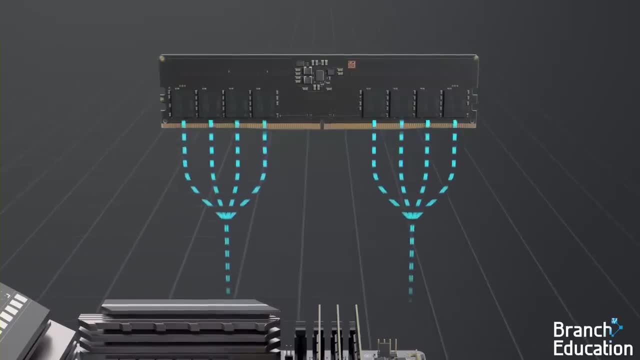 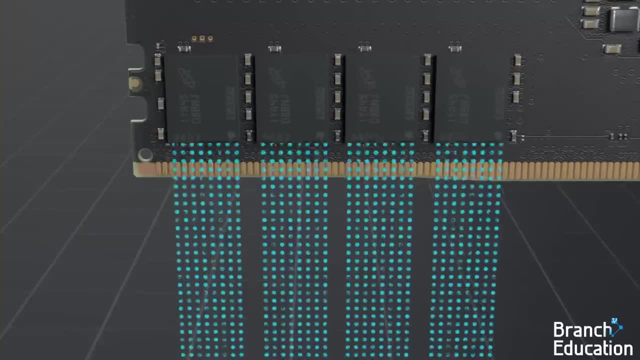 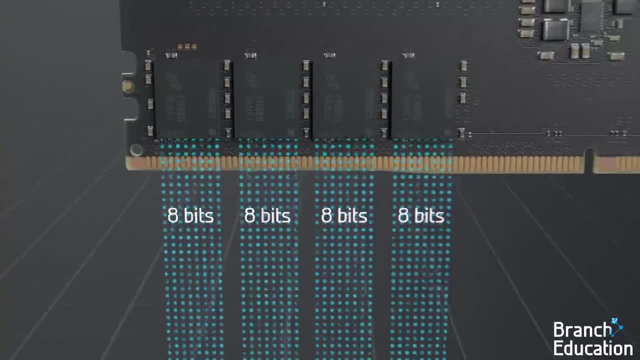 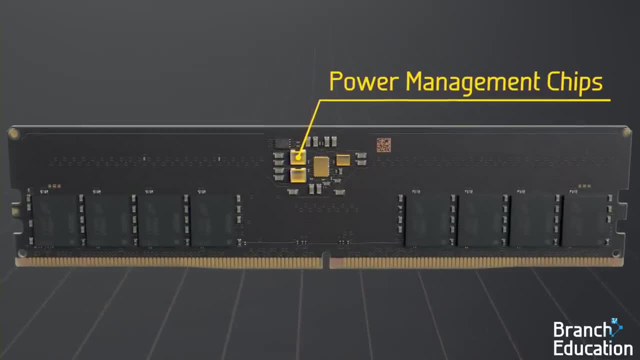 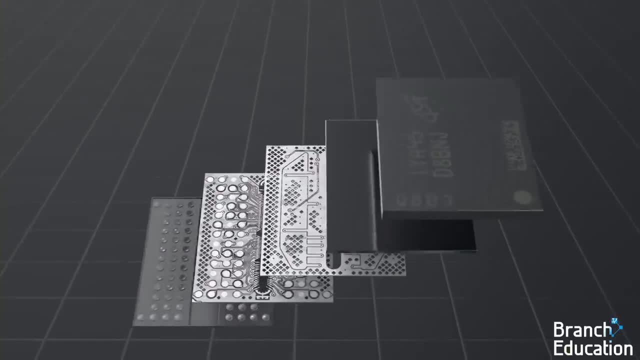 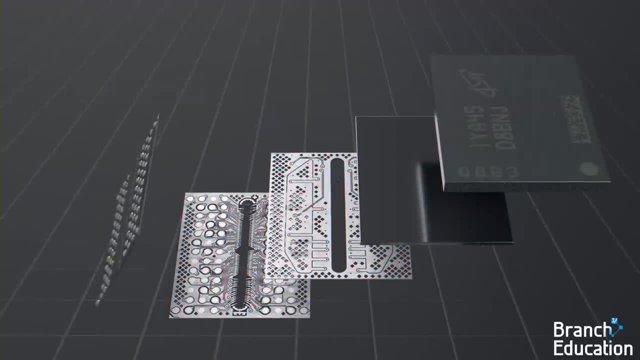 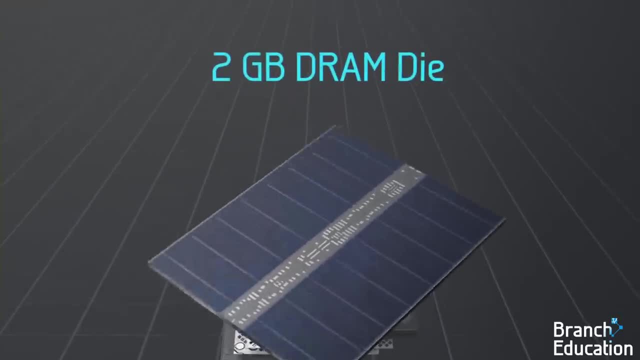 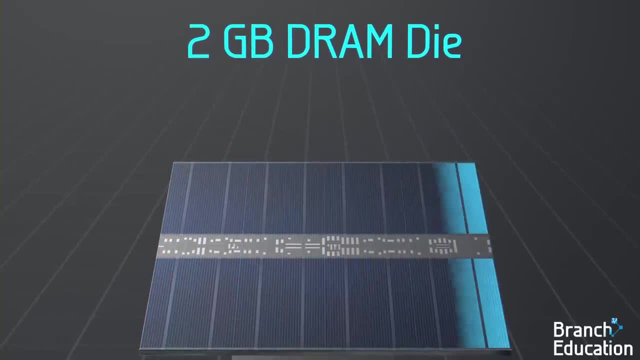 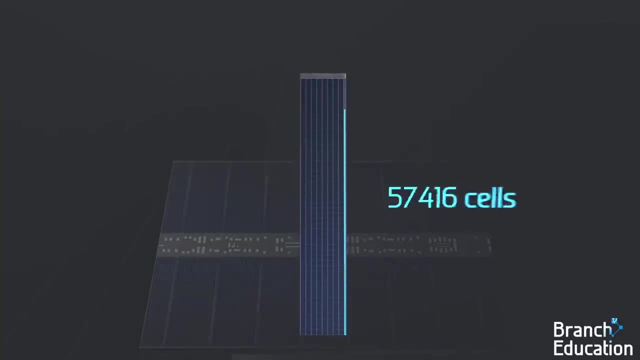 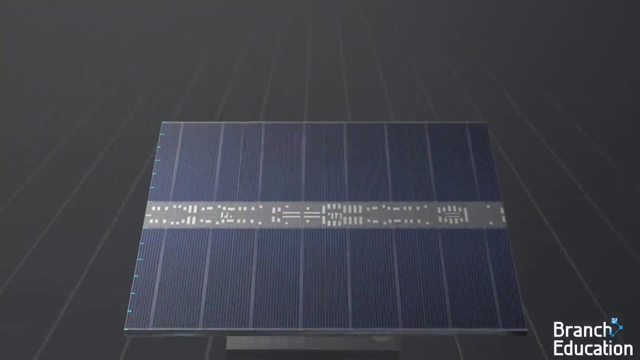 DRAM is limited to a single factor, composed of four banks, each totaling 32 banks. Within each bank is a massive array: 65,536 memory cells tall by 8,192 cells across, Essentially rows and columns in a grid. 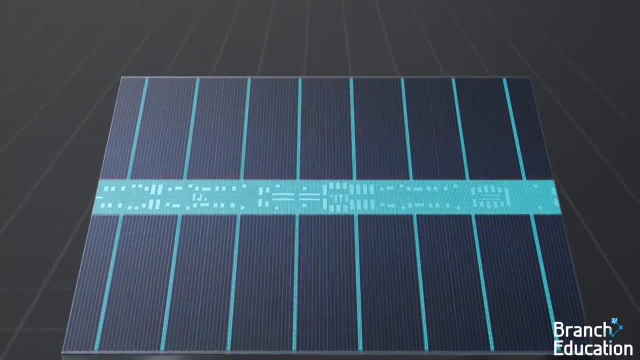 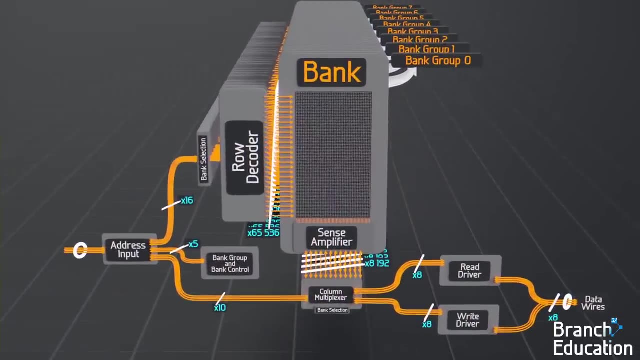 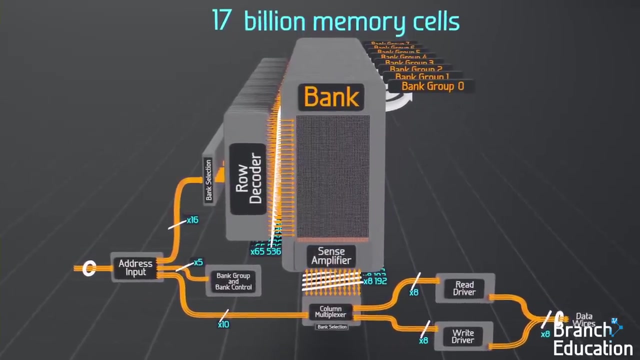 with tens of thousands of wires and supporting circuitry running outside each bank. Instead of looking at this die, we're going to transition to a functional diagram and then reorganize the banks and bank groups. In order to access 17 billion memory cells, we need a 31-bit address. 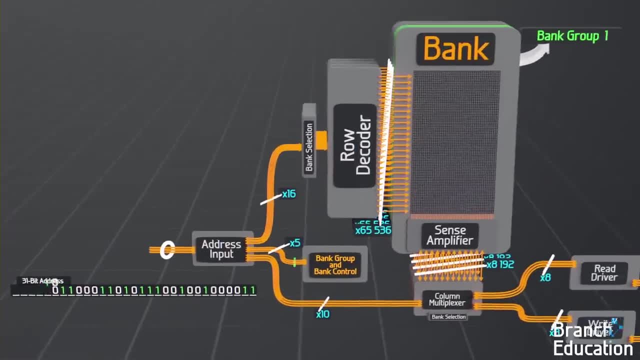 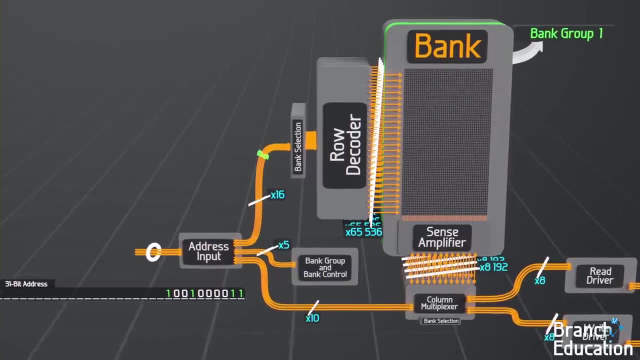 Three bits are used to select the appropriate bank group, then two bits to select the bank. Next, 16 bits of the address are used to determine the exact row out of 65,000.. Because this chip reads or writes 8 bits at a time. 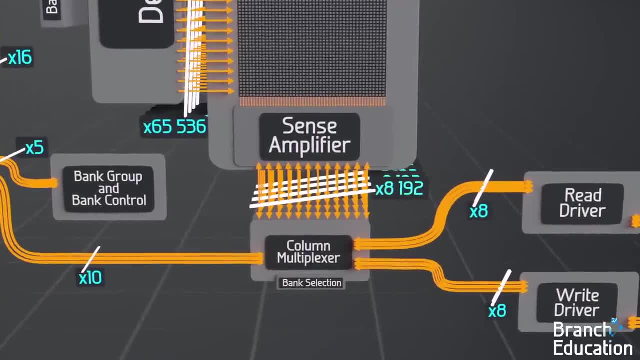 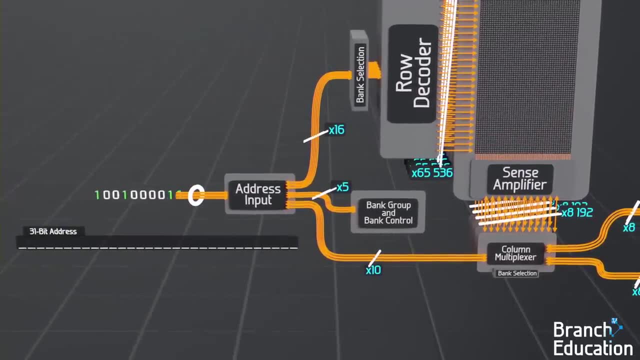 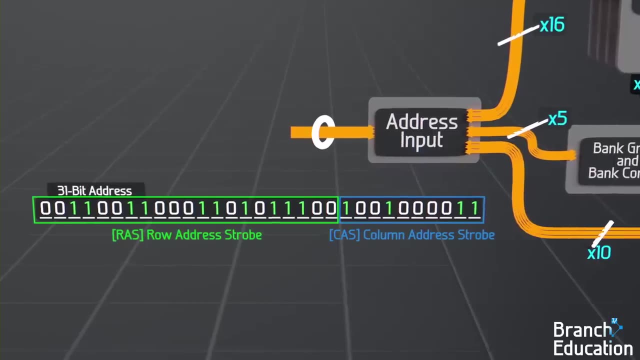 the 8,192 columns are grouped by 8 memory cells, all read or written at a time, or by 8. And thus only 10 bits are needed for the column address. One optimization is that this 31-bit address is separated into two parts and sent using only 21 wires. 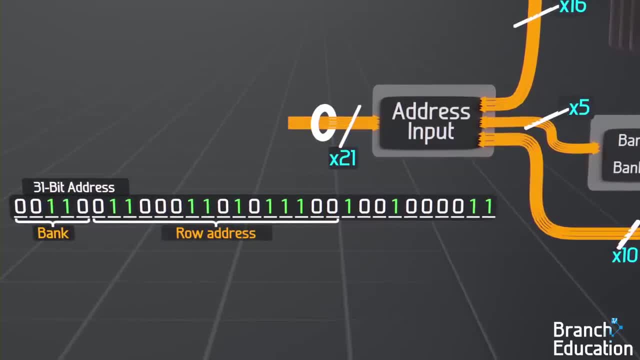 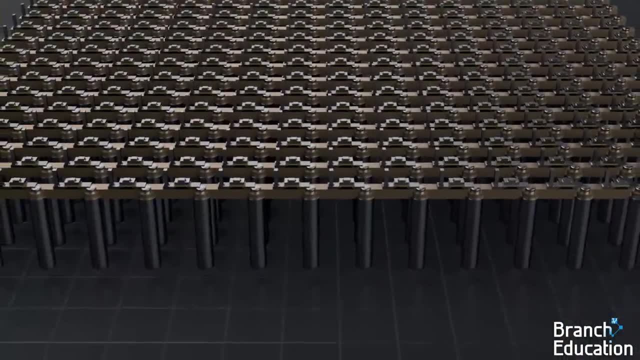 First the bank group, bank and row address are sent, and then, after that, the column address. Next we'll look inside these physical memory cells, But first let's briefly talk about how these structures are manufactured, as well as this video's sponsor. 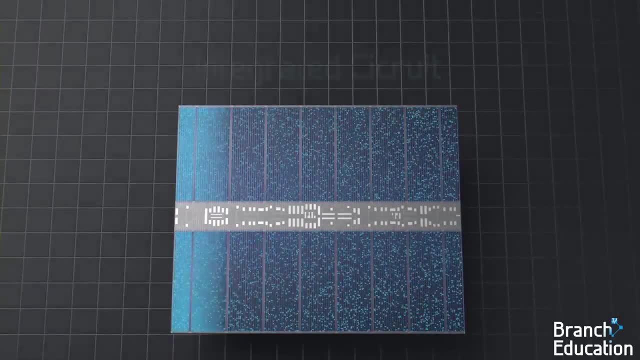 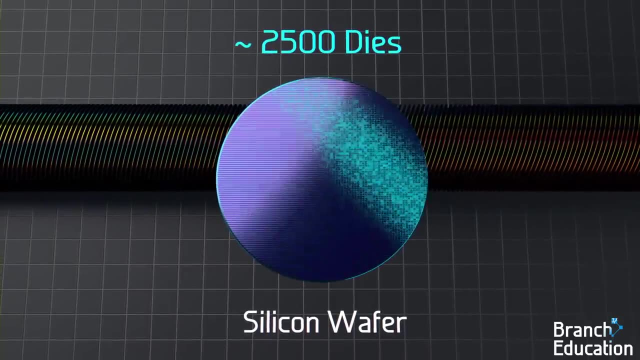 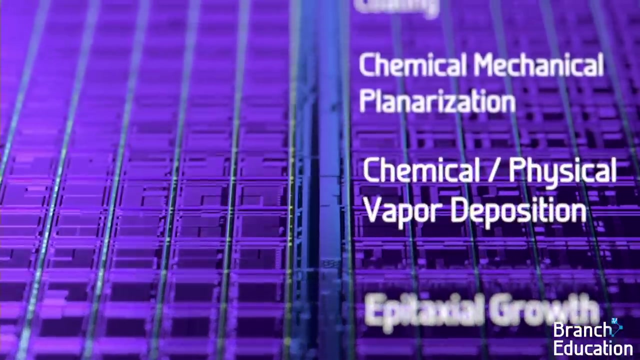 This incredibly complicated die, also called an integrated circuit, is manufactured on 300-millimeter silicon wafers, 2,500-ish dies at a time. On each die are billions of nonoscopic memory cells that are fabricated using dozens of tools and hundreds of steps. 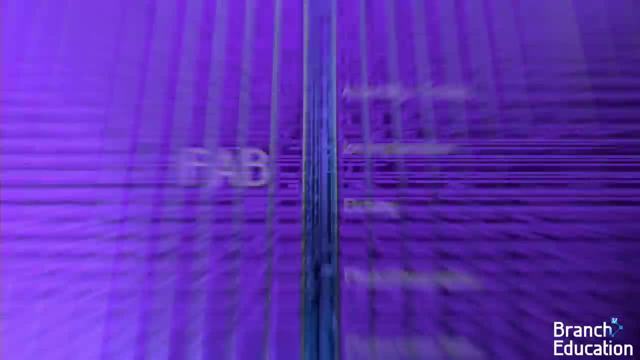 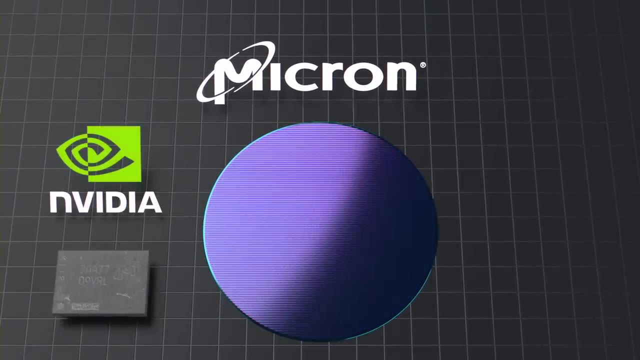 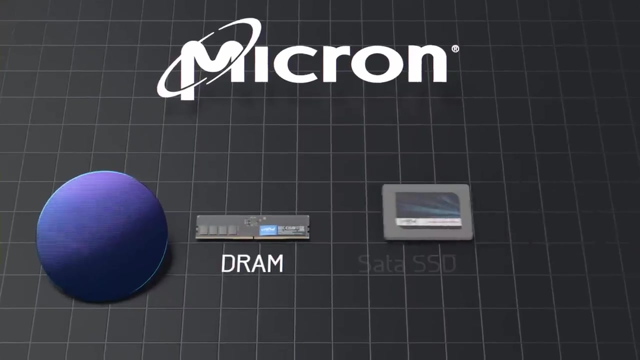 in a semiconductor fabrication plant, or FAB. This one was made by, which manufactures around a quarter of the world's DRAM, including both NVIDIA's and AMD's VRAM in their GPUs. Micron also has its own product line of DRAM and SSDs under the brand Crucial. 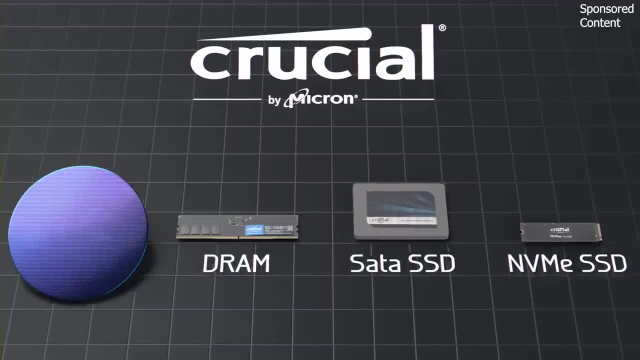 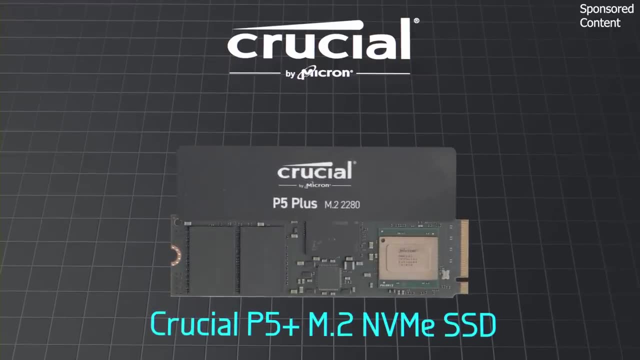 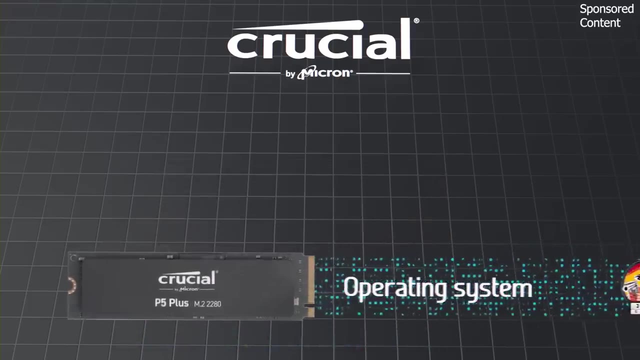 which, as mentioned earlier, is the sponsor of this video. In addition to DRAM, Micron is one of the world's leading suppliers of solid-state drives such as this Crucial P5 Plus M2 NVMe SSD. By installing your operating system in video games on a Crucial NVMe solid-state drive. 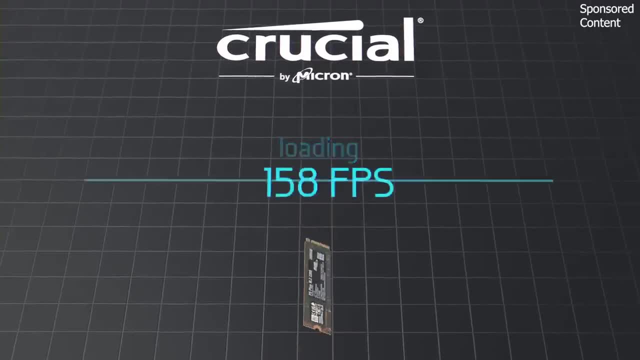 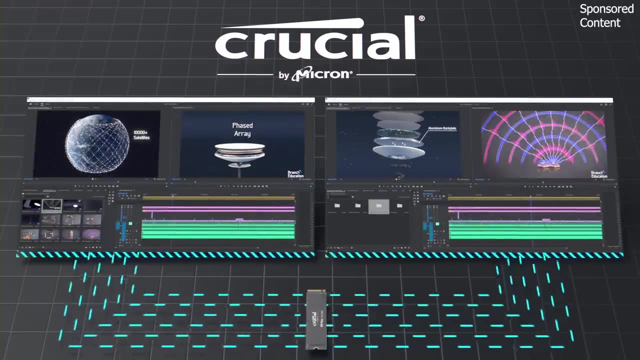 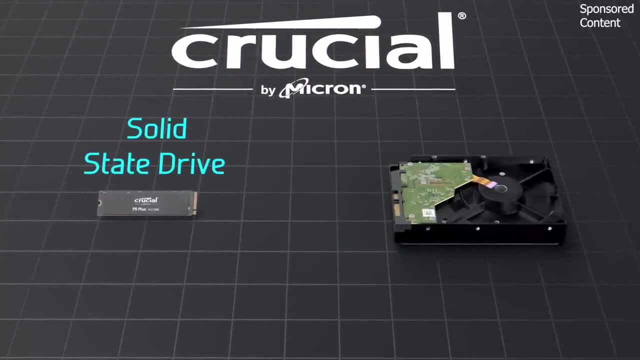 you'll be sure to have incredibly fast loading times and smooth gameplay. And if you do video editing, make sure all those files are on a fast SSD like this one as well. This is because the main speed bottleneck for loading is predominantly limited by the speed of the SSD or hard drive where the files are stored. 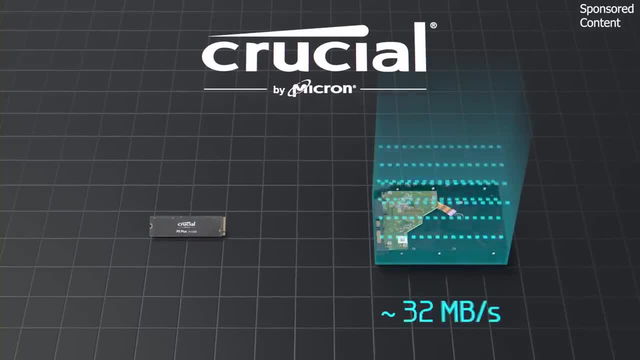 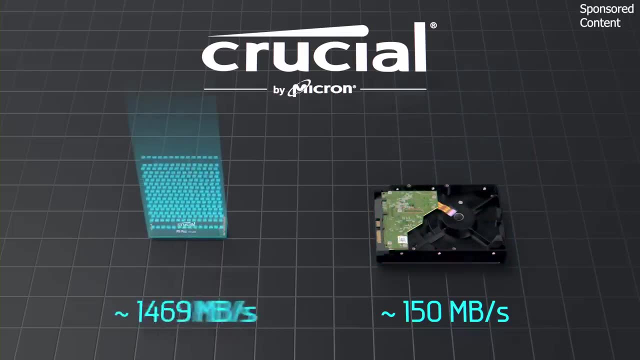 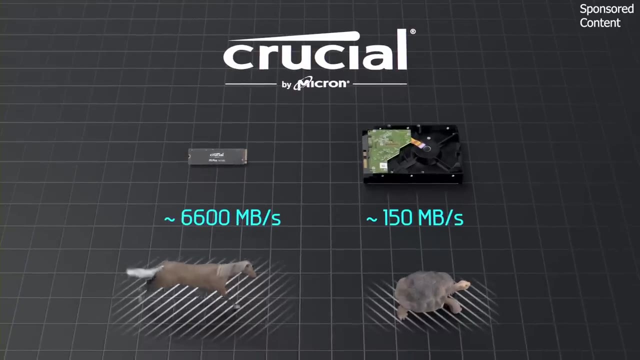 For example, this hard drive can only transfer data at around 150 megabytes a second, whereas this Crucial NVMe SSD can transfer data at a rate of up to 6,600 megabytes a second, which, for comparison, is the speed of a moving tortoise versus a galloping horse. 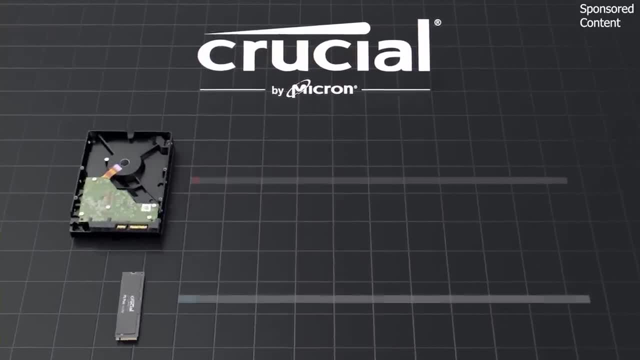 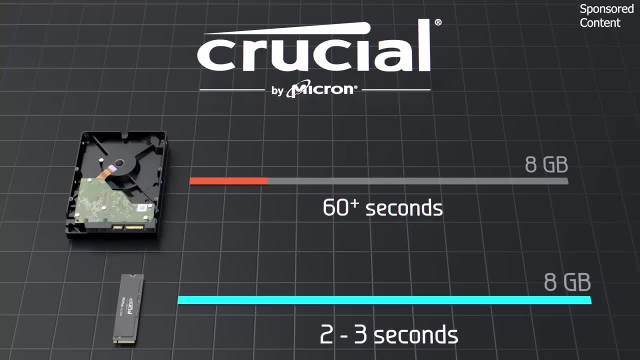 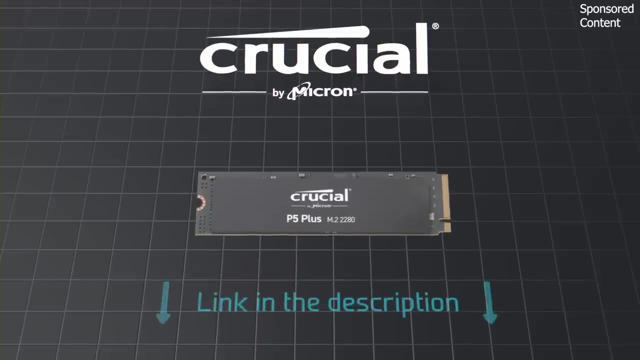 By using a Crucial NVMe SSD, loading a video game that requires gigabytes of DRAM is reduced from a minute or more down to a couple of seconds. Check out the Crucial NVMe SSDs using a link in the description below. 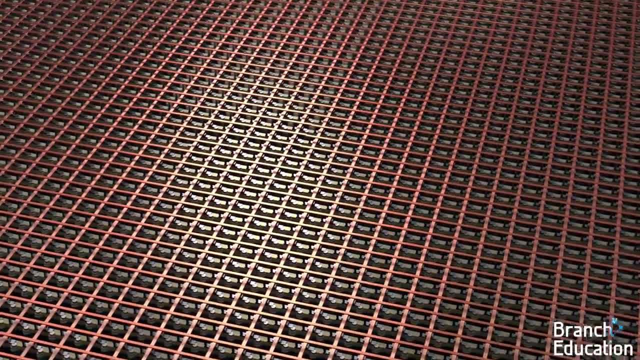 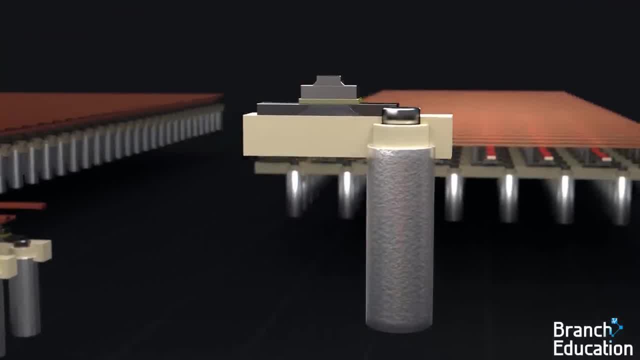 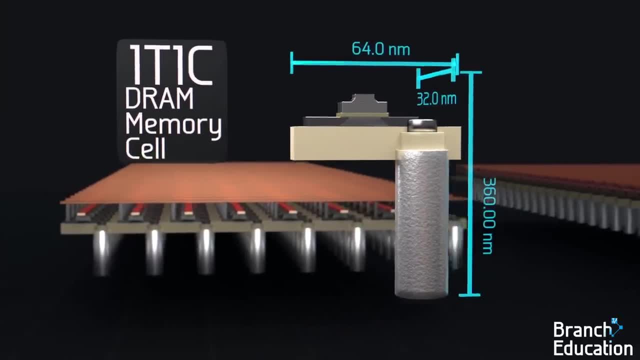 Let's get back to the details of how DRAM works and zoom in to explore a single memory cell situated in a massive array. This memory cell is called a 1T1C cell and is a few dozen nanometers in size. It has two parts. 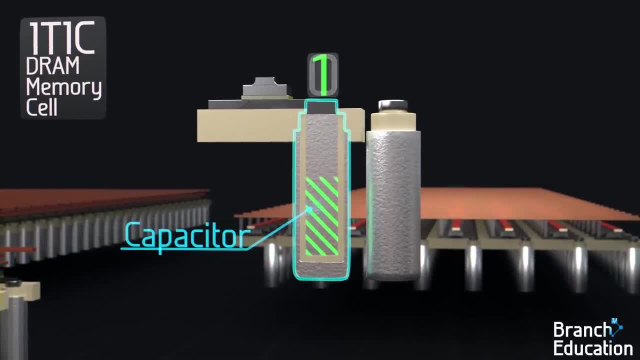 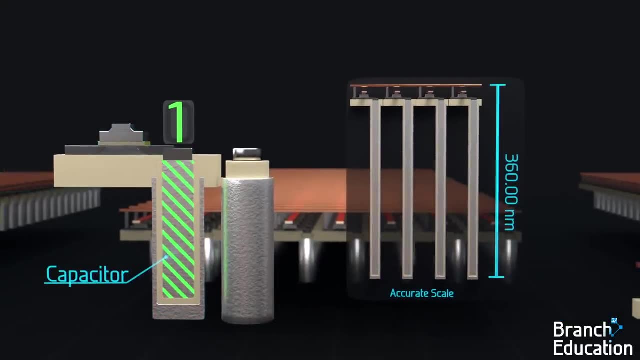 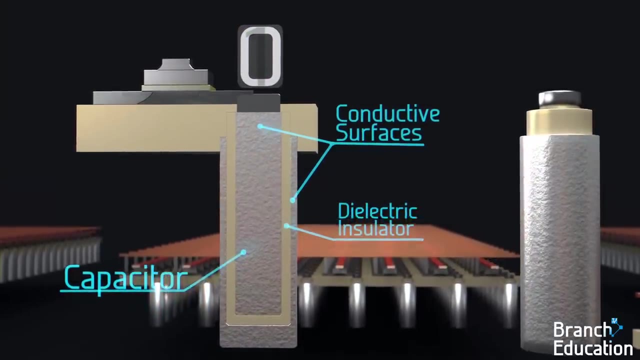 It stores one bit of data in the form of electrical charges or electrons and a transistor to access and read or write data. The capacitor is shaped like a deep trench dug into silicon and is composed of two conductive surfaces separated by a dielectric insulator or barrier just a few atoms thick. 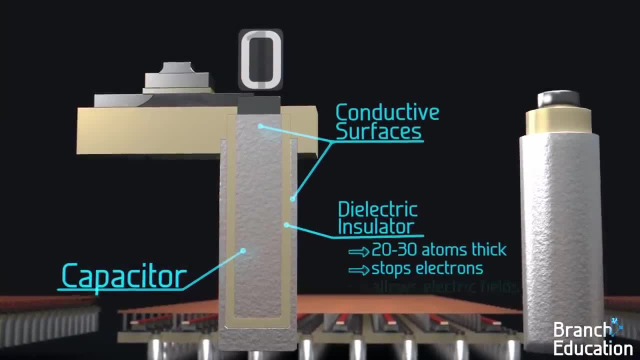 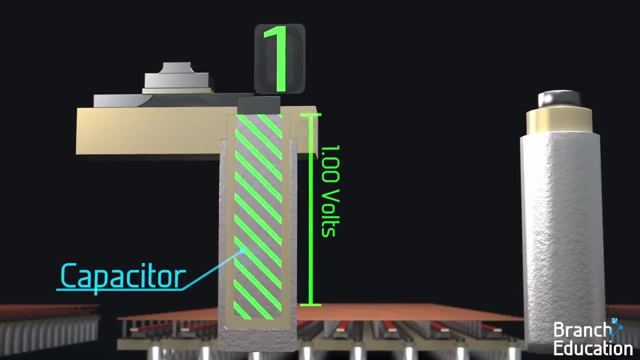 which stops the flow of electrons but allows electric fields to pass through. If this capacitor is charged up with electrons to one volt, it's a binary one, And if no charges are present and it's at zero volts, it's a binary zero. 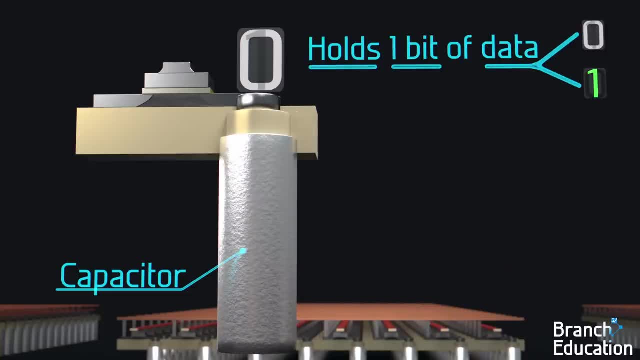 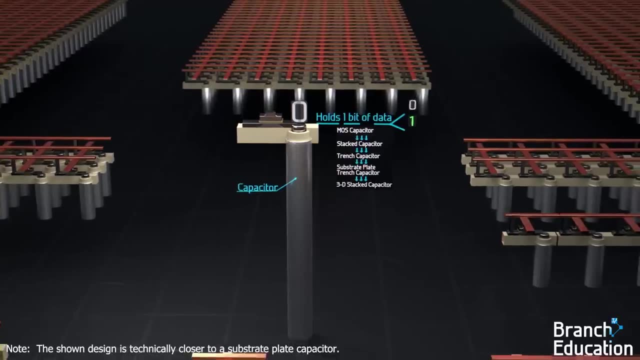 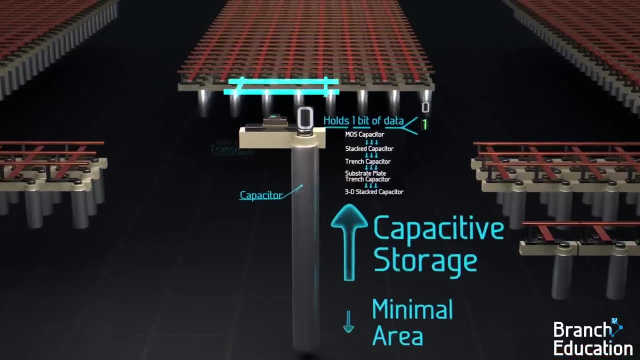 And thus this cell only holds one bit of data. Designs of capacitors are constantly evolving, but in this trench capacitor, the depth of the silicon is utilized to allow for larger capacitive storage while taking up as little area as possible. Next, let's look at the access transistor and add in two wires. 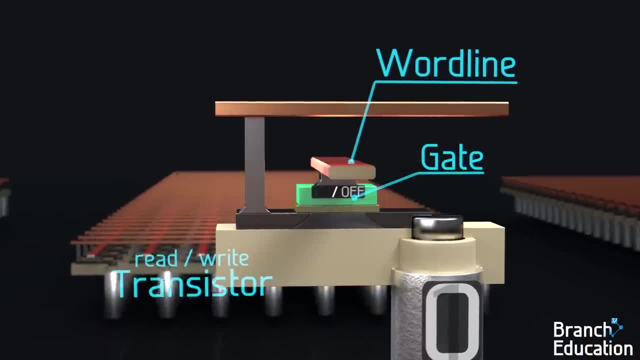 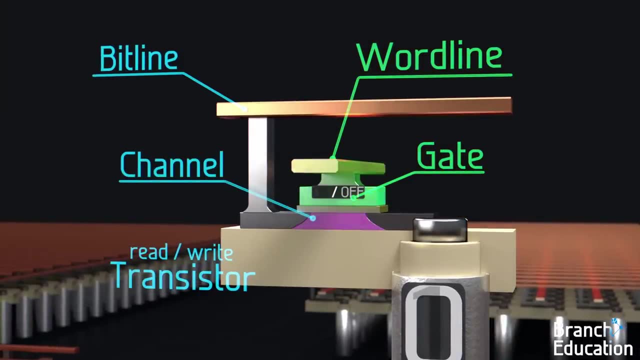 The wordline wire connects to the gate of the transistor, while the bitline wire connects to the other side of the transistor's channel. Applying a voltage to the wordline turns on the transistor and while it's on, electrons can flow through the channel. 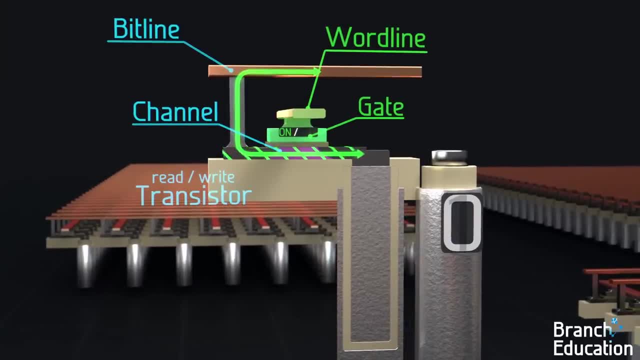 thus connecting the capacitor to the bitline. This allows us to access and charge up the capacitor to write a one, or discharge the capacitor to write a zero. Additionally, we can read the stored value in the capacitor by measuring the amount of charge. However, when the wordline is off, the transistor is turned off. 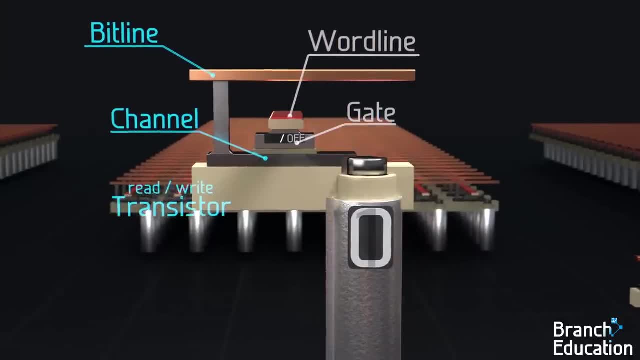 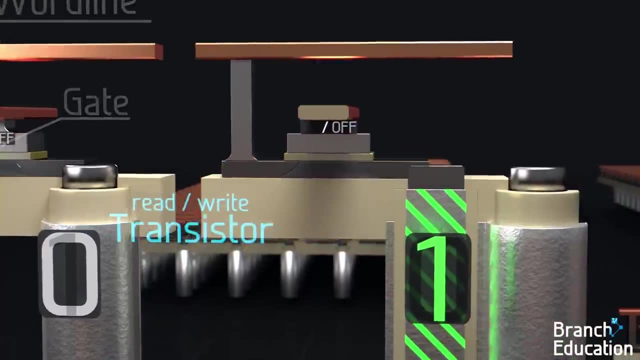 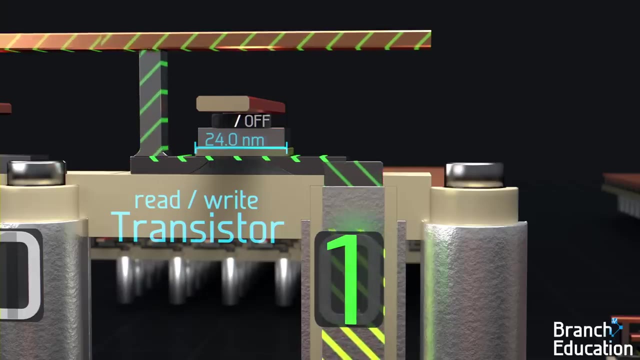 and the capacitor is isolated from the bitline, thus saving the data or charge that was previously written. Note that because this transistor is incredibly small, only a few dozen nanometers wide, electrons slowly leak across the channel and thus, over time, the capacitor needs to be refreshed. 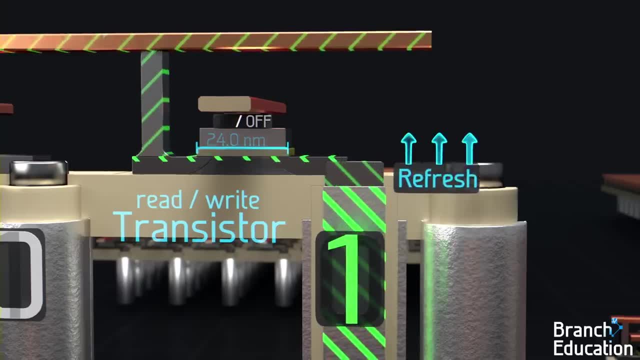 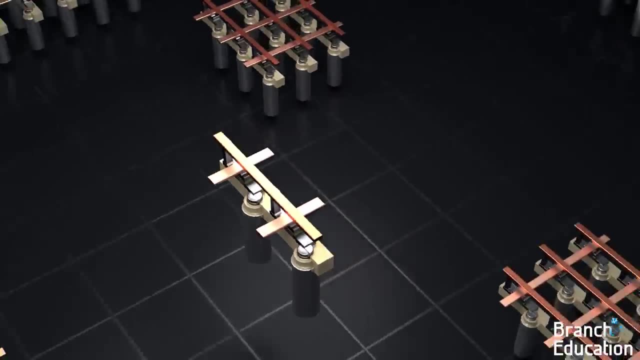 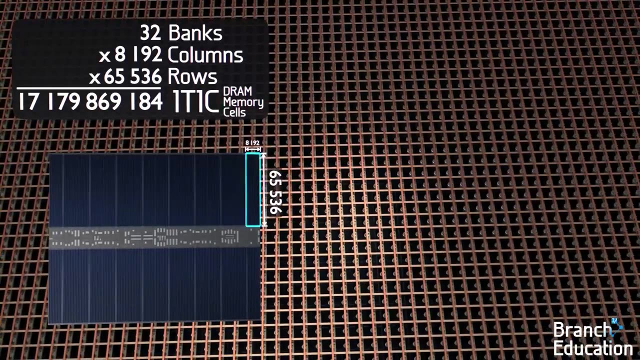 to recharge the leaked electrons. We'll cover exactly how refreshing memory cells works a little later. As mentioned earlier, this 1T1C memory cell is one of 17 billion inside this single die and is organized into massive arrays called banks. 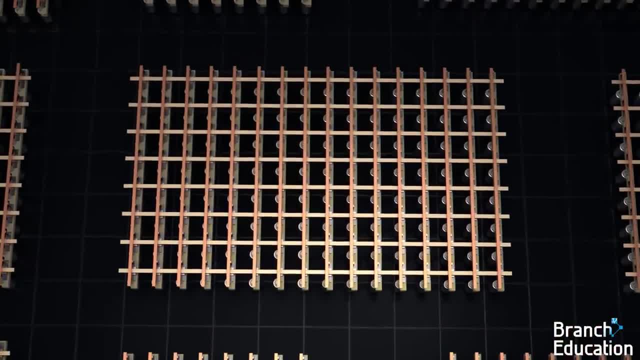 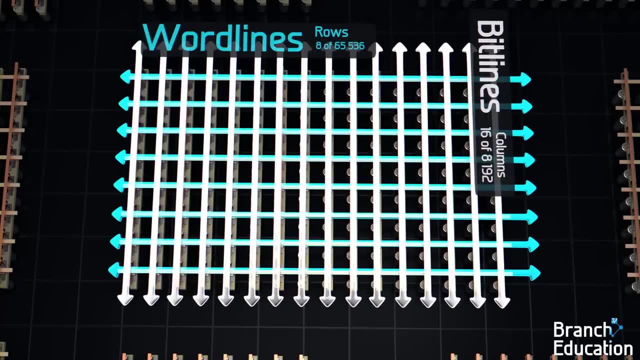 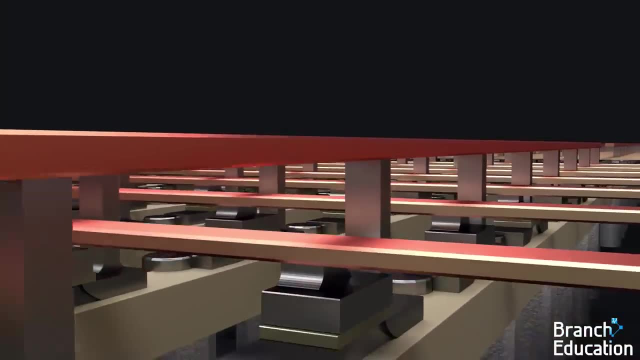 So let's build a small array for illustrative purposes. In our array each of the wordlines is connected in rows and then the bitlines are connected in columns. Wordlines and bitlines are in different vertical layers, so one can cross over the other and they never touch. 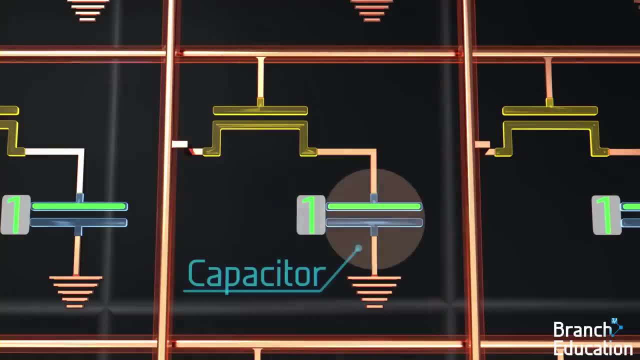 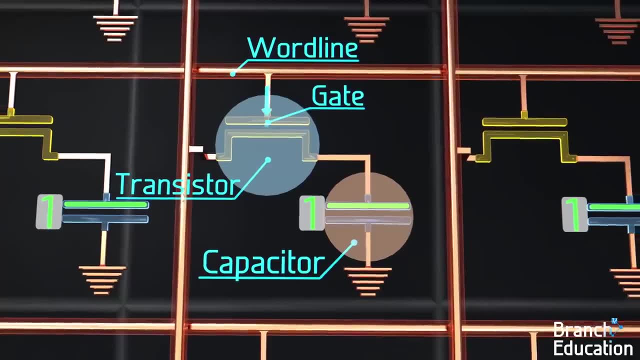 Let's simplify the visual and use symbols for the capacitors and the transistors. Just as before, the wordlines connect to each transistor's control gate in rows, and then all the bitlines in columns connect to the channel opposite each capacitor. 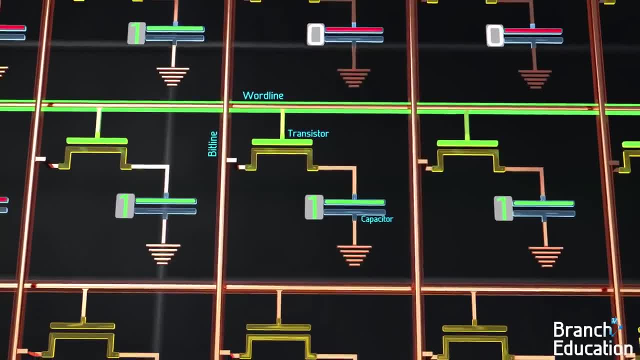 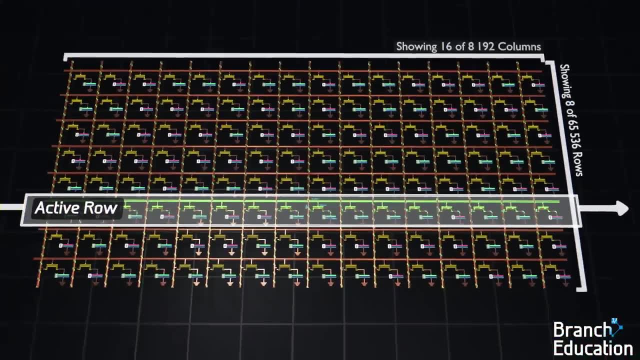 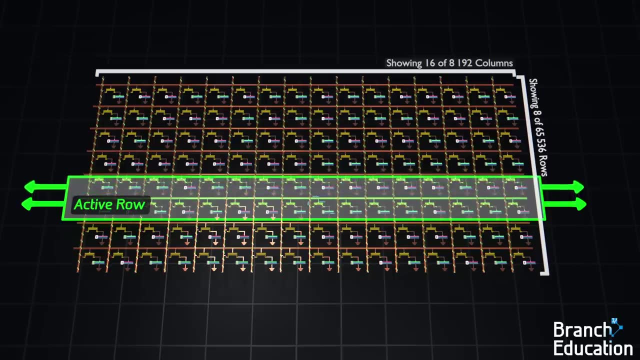 As a result, when a wordline is active, all the capacitors in only that row are connected to their corresponding bitlines, thereby activating all the memory cells in that row. At any given time, only one wordline is active, because if more than one wordline were active, 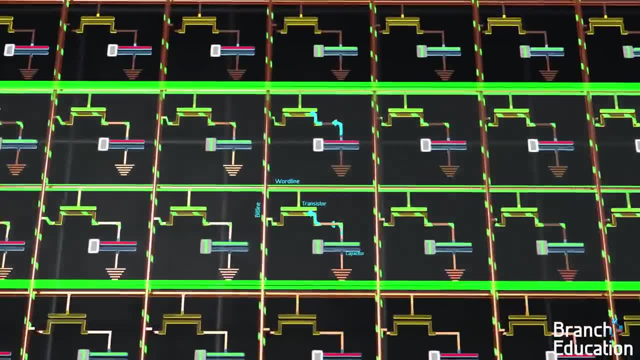 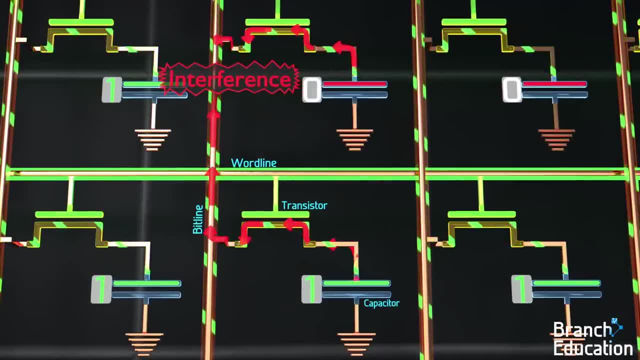 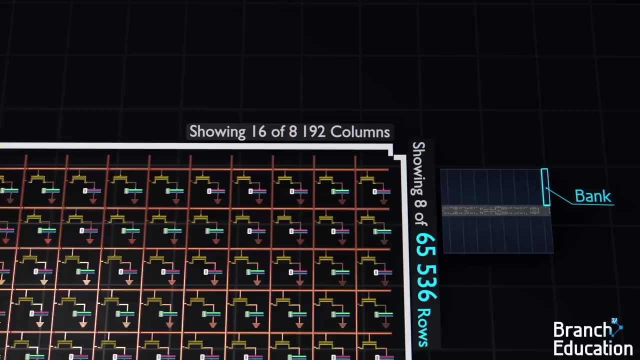 then multiple capacitors in a column would be connected to the bitline and the data storage functionalities of these capacitors would interfere with one another, making them useless. As mentioned earlier, within a single bank there are 65,536 rows and 8,192 columns. 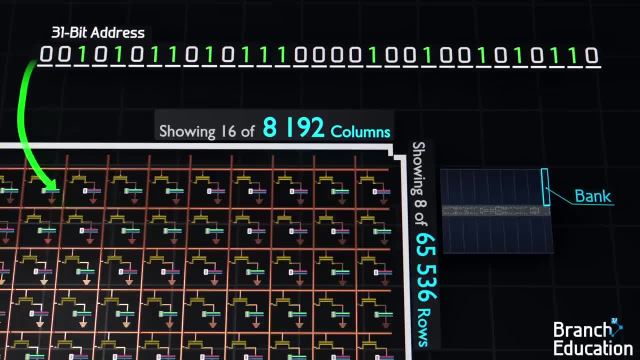 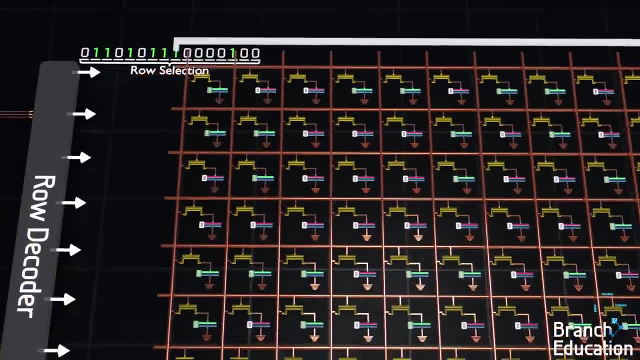 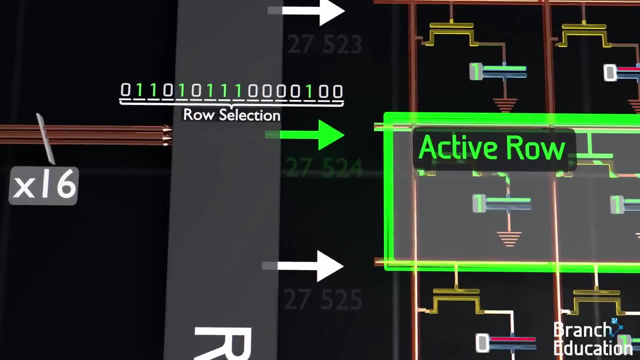 and the 31-bit address is used to activate a group of just eight memory cells. The first five bits select the bank and the next 16 bits are sent to a row decoder to activate a single row. For example, this binary number turns on the wordline row 27,524,. 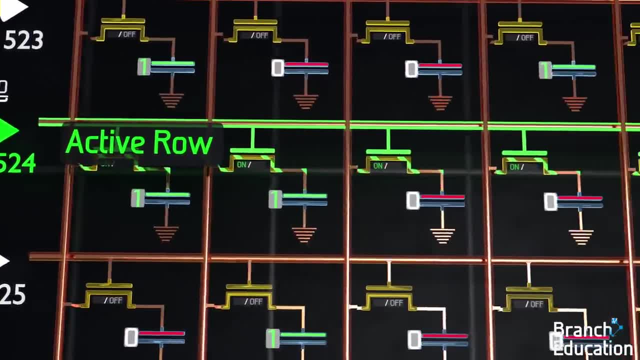 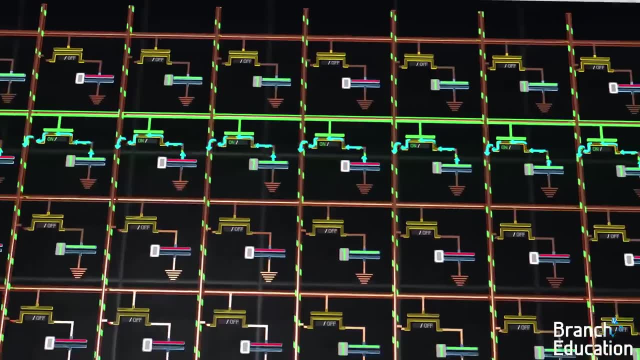 thus turning on all transistors in the bank By connecting the eight-thousand-192 in that row and connecting the 8,192 capacitors to their bitlines, while at the same time the other 65thousandish wordlines are all off. 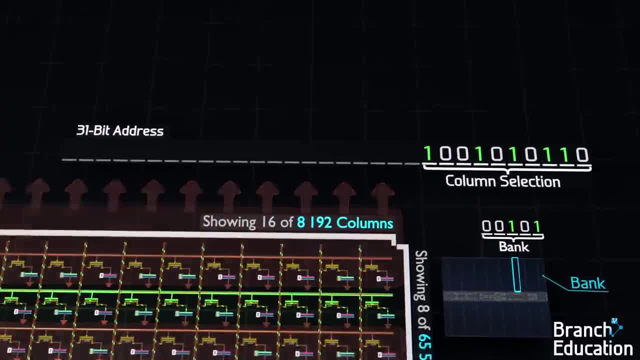 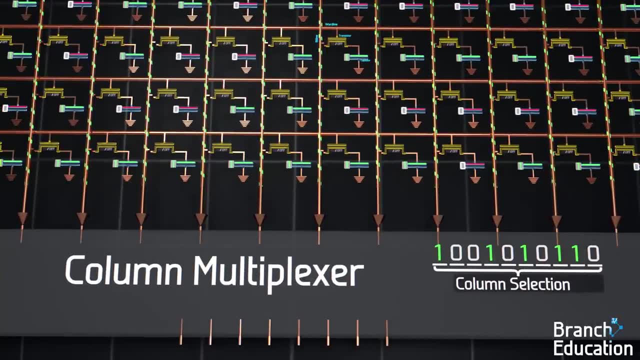 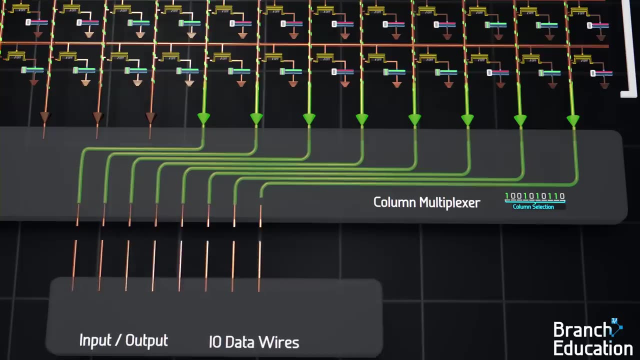 Here's the logic diagram for a simple decoder. The remaining ten bits of the address are sent to the column multiplexer. This multiplexer takes in the 8,192 bitlines on the top and, depending on the ten-bit address lines to the 8 input and output I-O wires at the bottom. For example, if the 10-bit address were: 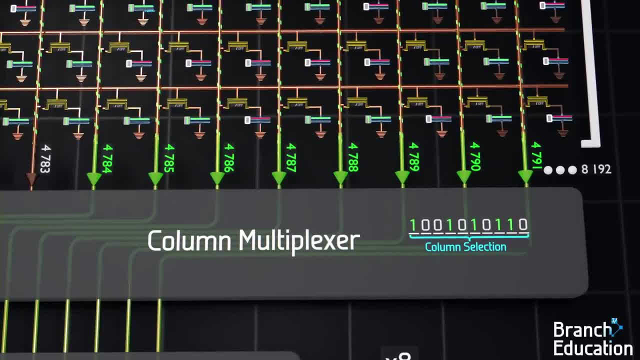 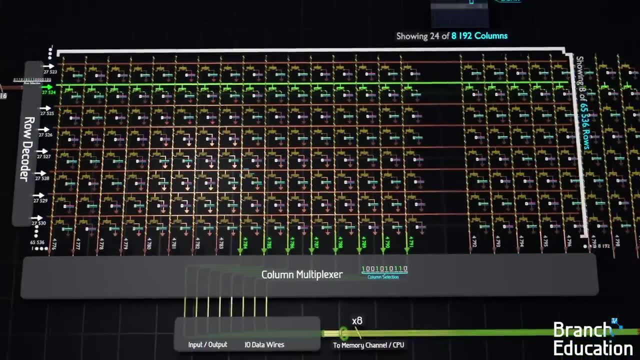 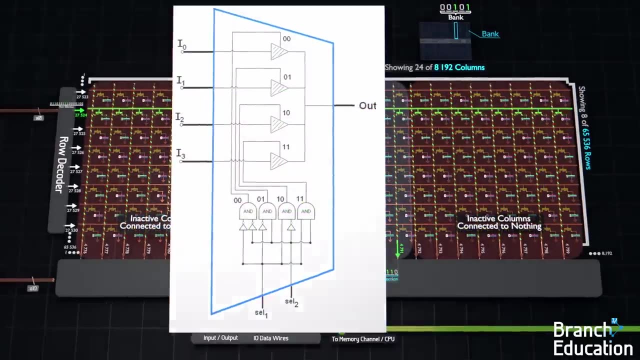 this, then only the bit lines 4784 through 4791 would be connected to the I-O wires and the rest of the 8000-ish bit lines would be connected to nothing. Here's the logic diagram for a simple multiplexer. We now have the means of accessing any memory cell in this massive array. However, 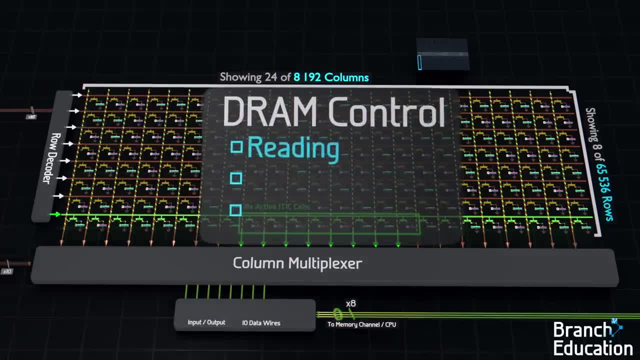 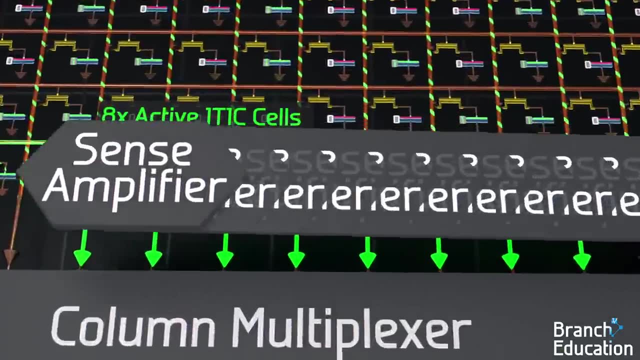 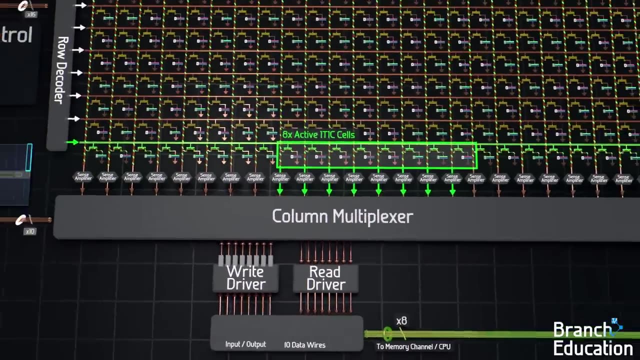 to understand the three basic operations: reading, writing and refreshing. let's add two elements to our layout: A sense amplifier at the bottom of each bit line and a read and write driver outside of the column multiplexer. Let's look at reading from a group of memory cells. First, the read command. 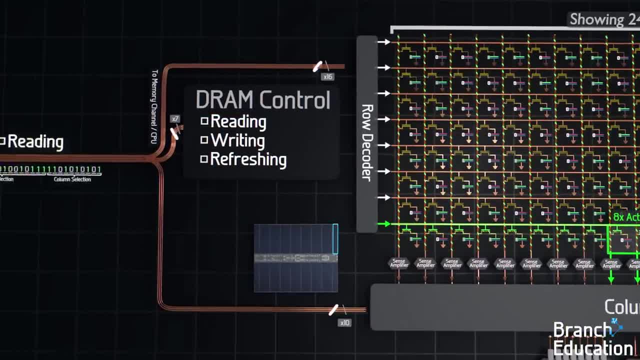 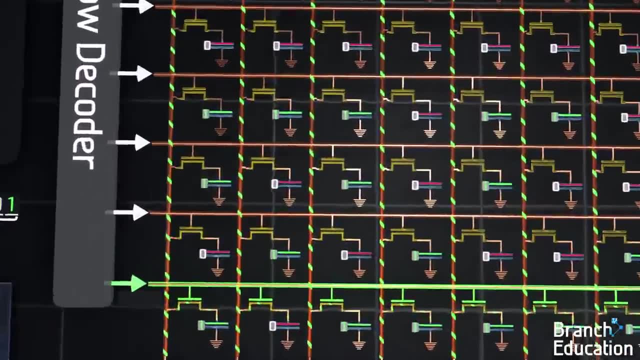 and 31-bit address are sent from the CPU to the DRAM. The first five bits select a specific bank. The next step is to turn off all the word lines in that bank, thereby isolating all the capacitors, and then pre-charge all 8000-ish. 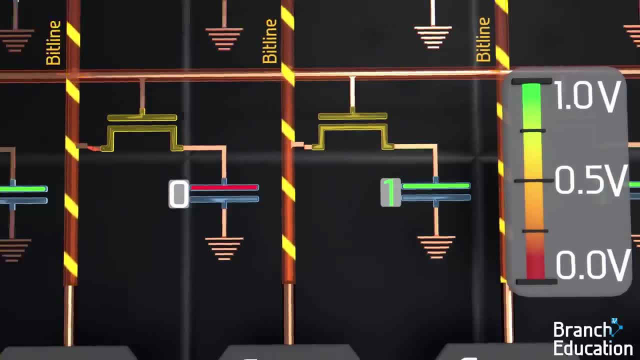 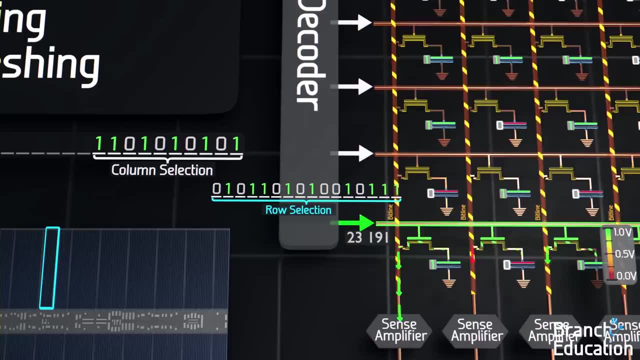 bit lines to 0.5 volts. Next the 16-bit row address turns on a row and all the capacitors in that row are connected to their bit lines. If an individual capacitor holds a 1 and is charged to 1 volt. 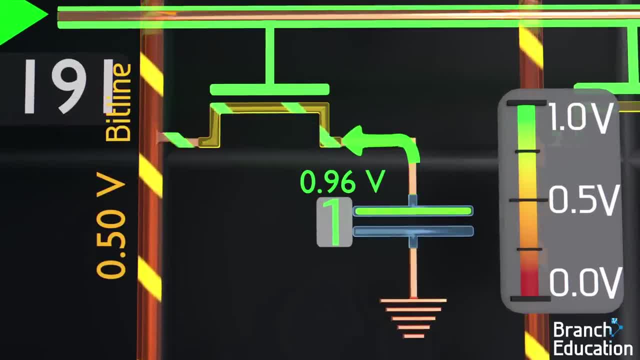 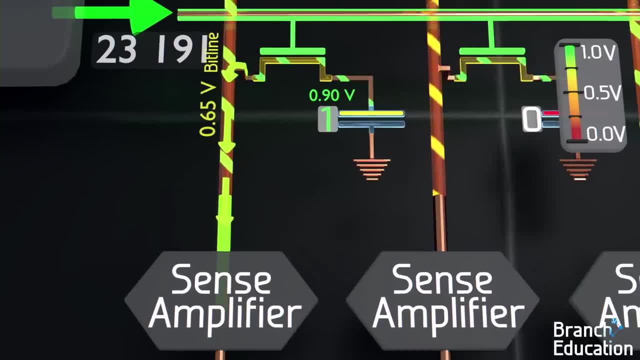 then some charge flows from the capacitor onto the 0.5 volt bit line and the voltage on the bit line decreases. The sense amplifier then detects the slight change or perturbation of voltage on the bit line, amplifies the change and pushes the voltage on the bit line all the way up to 1 volt. However, 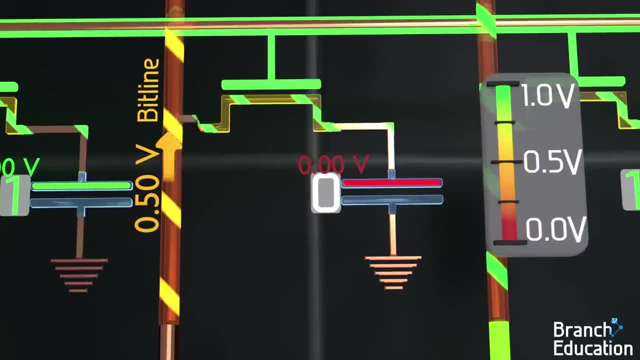 if a 0 is stored in the capacitor, charge flows from the bit line into the capacitor and the 0.5 volt bit line decreases in voltage. The sense amplifier then sees this change, amplifies it and drives the bit line voltage down to 0 volts or 0.5 volts. 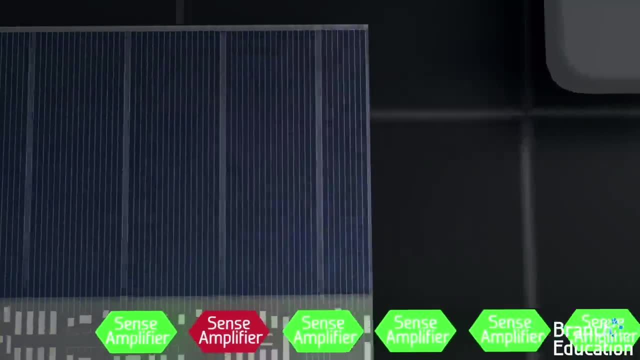 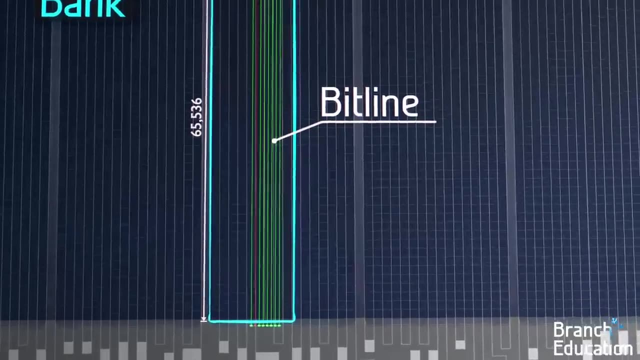 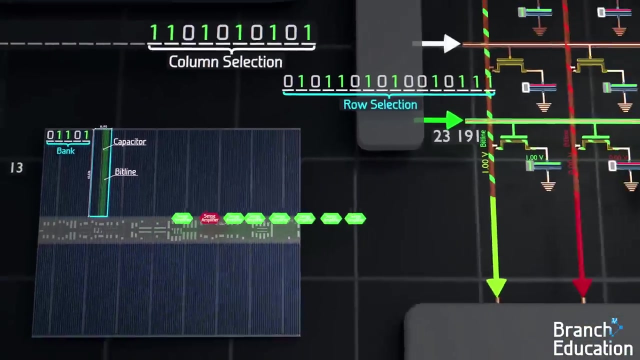 The sense amplifier is necessary because the capacitor is so small and the bit line is rather long, and thus the capacitor needs to have an additional component to sense and amplify whatever value is stored. Now all 8000-ish bit lines are driven to 1 volt or 0 volts, corresponding to the stored charge in the 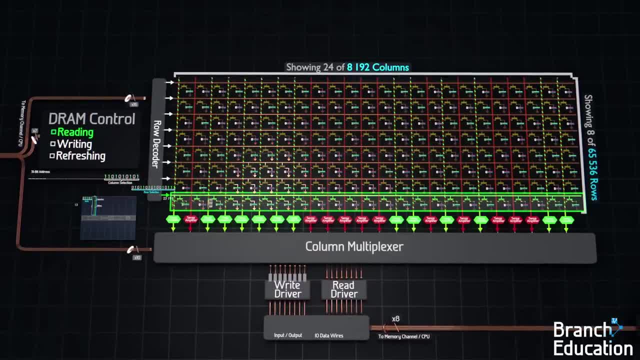 capacitors of the activated row, and this row is now considered open. Next, the column select multiplexer uses the 0.5 volt bit line to control the voltage in the capacitor and the 0.5 volt bit line to control the voltage in the capacitor. 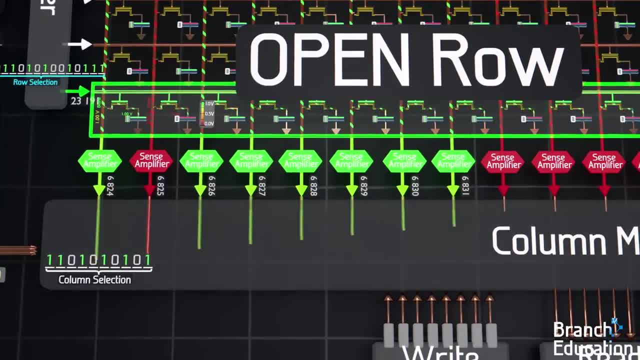 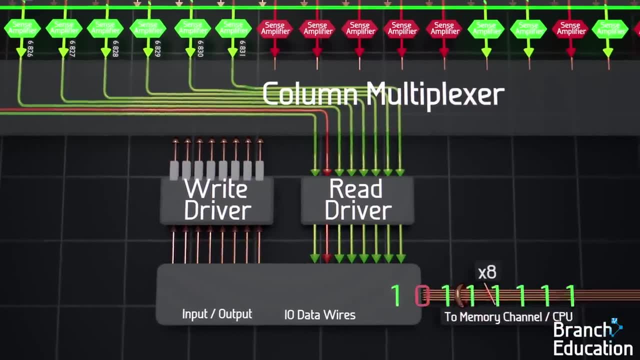 Next the 10-bit column address to connect the corresponding 8-bit lines to the read driver, which then sends these 8 values and voltages over the 8 data wires to the CPU. Writing data to these memory cells is similar to reading. 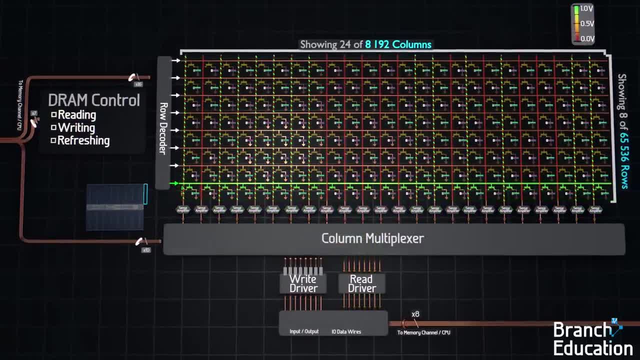 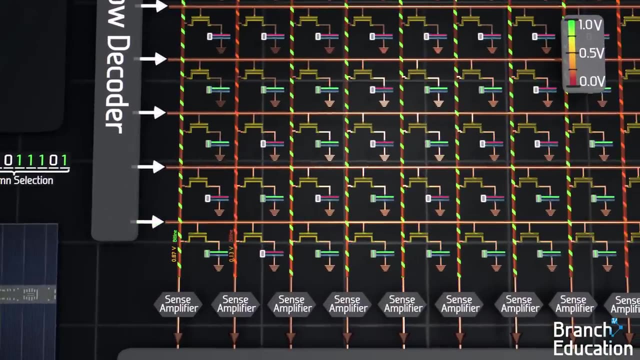 however, with a few key differences. First, the write command address and 8 bits to be written are sent to the DRAM chip. Next, just like before the bank is selected, the capacitors are isolated and the bit lines are pre-charged to 0.5 volts. Then, using a 16-bit, 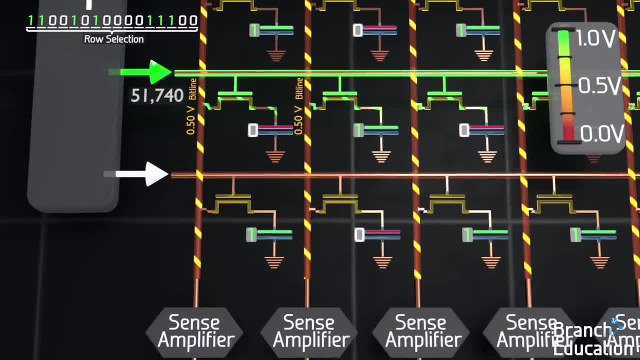 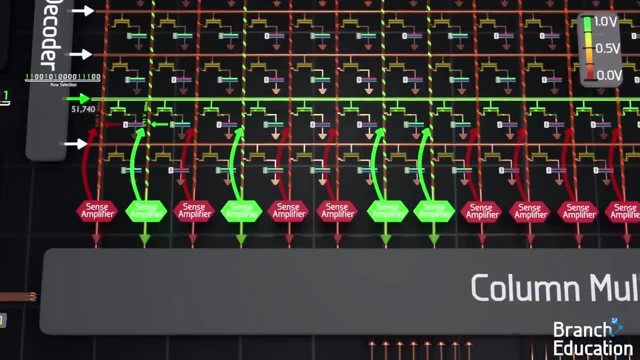 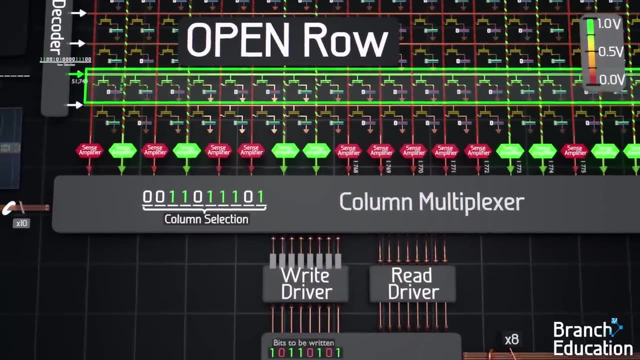 address, a single row is activated, the capacitors perturb the bit line and the sense amplifiers sense this and drive the bit lines to a 1, or 0,, thus opening the row. Next, the column address goes to the multiplexer, but this time, because a write command was sent, the multiplexer connects the specific 8-bit line to the SDDR. 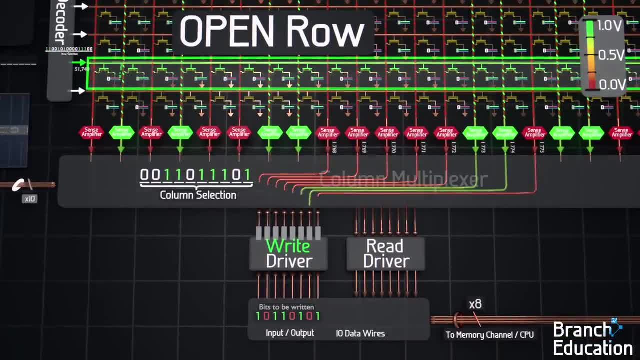 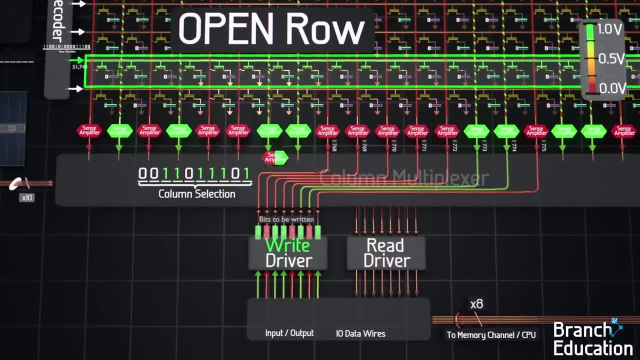 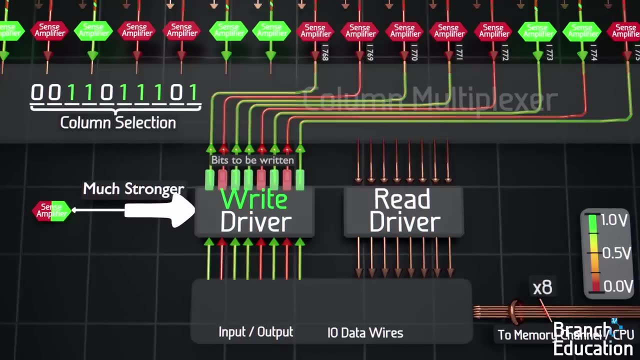 connects the specific 8-bit lines to the write driver, which contains the 8 bits that the CPU had sent along the data wires and requested to write. These write drivers are much stronger than the sense amplifier and thus they override whatever voltage was previously on the bit line and drive each of the 8-bit. 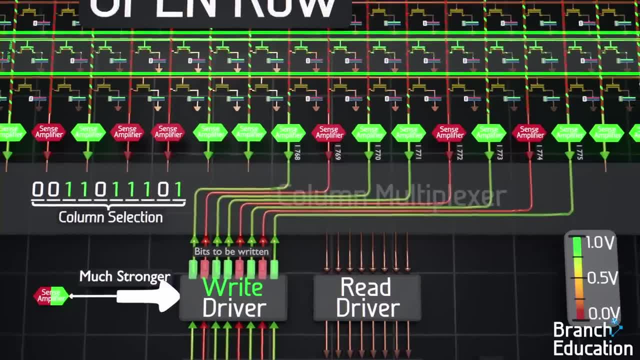 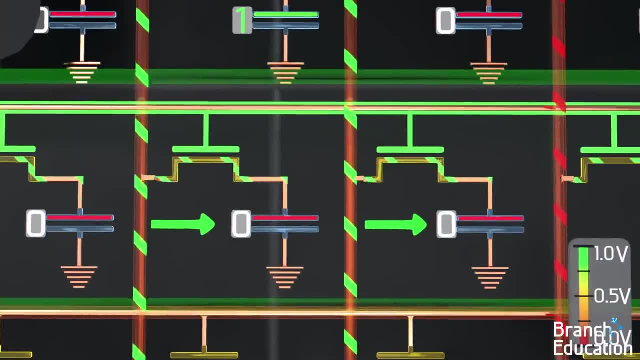 lines to 1 volt for a 1 to be written or 0 volts for a 0.. This new bit line voltage overrides the previously stored charges or values in each of the 8 capacitors in the open row, thereby writing 8 bits of data to the memory. 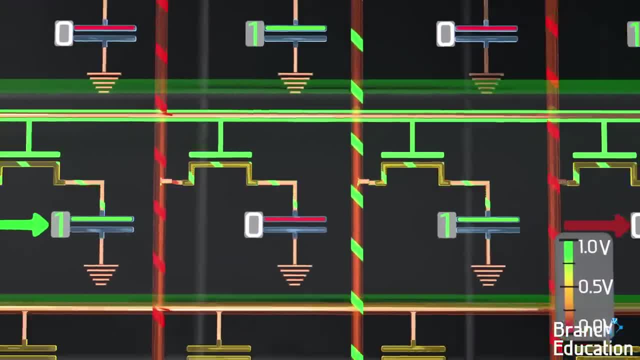 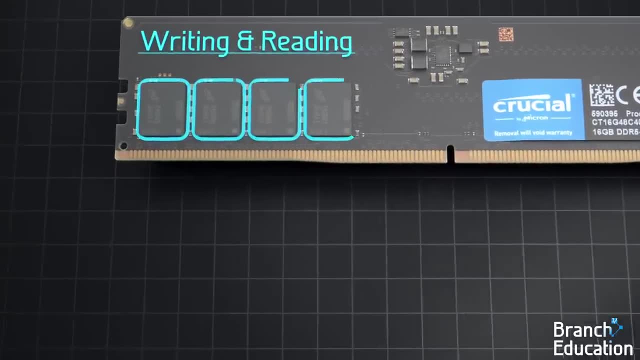 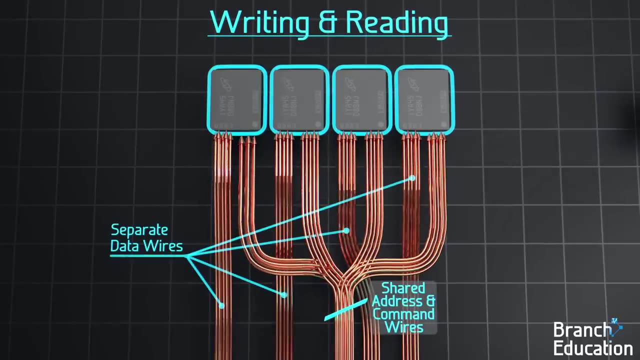 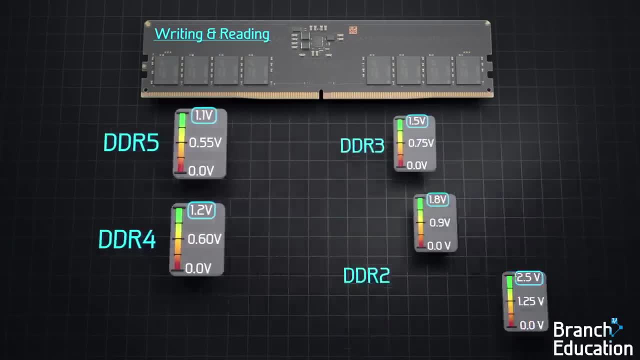 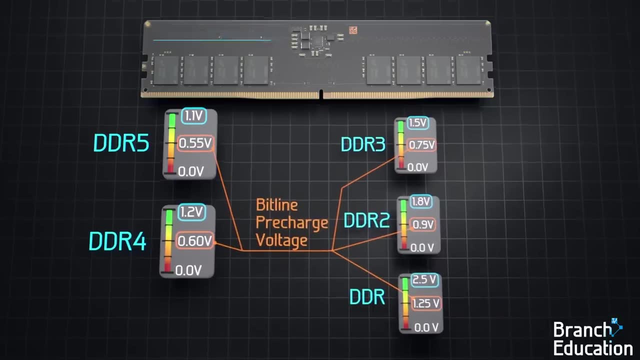 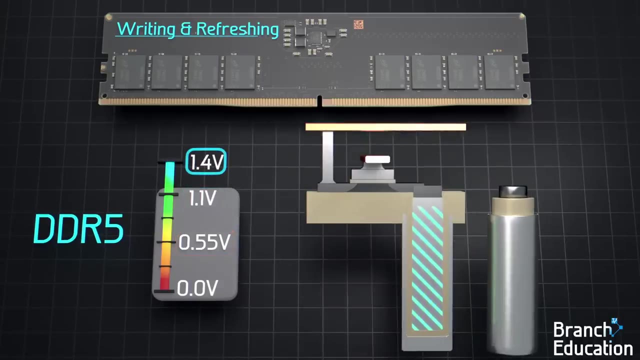 For DDR4, it's 1.2 volts, And prior generations had even higher voltages, with the bit line pre-charge voltages being half of these voltages. However, for DDR5, when writing or refreshing, a higher voltage, around 1.4 volts, is applied, and 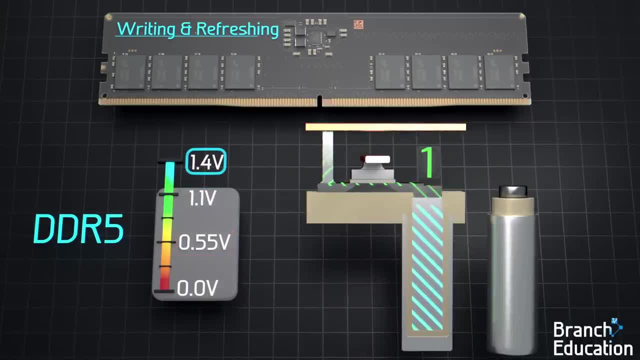 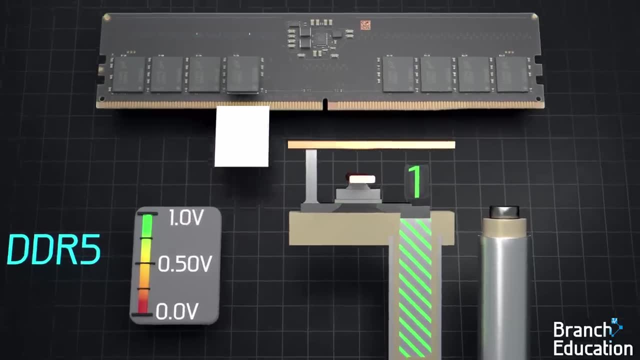 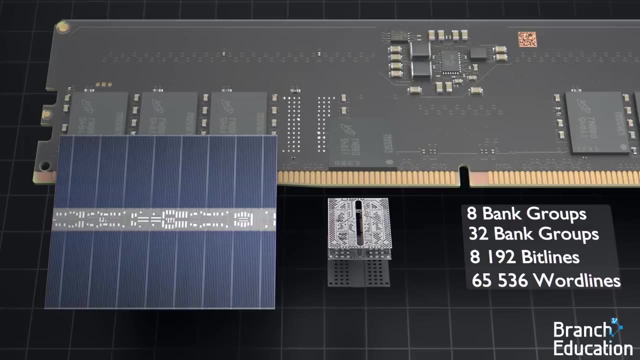 stored in each capacitor for a binary 1 because charge leaks out over time. However, for simplicity we're going to stick with 1 and 0.. Third, the number of bank groups, banks, bit lines and word lines varies widely between different generations and. 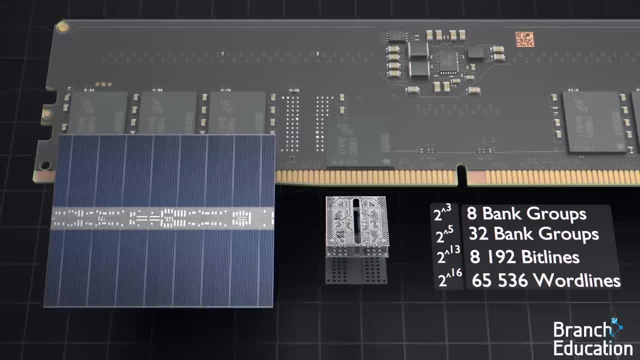 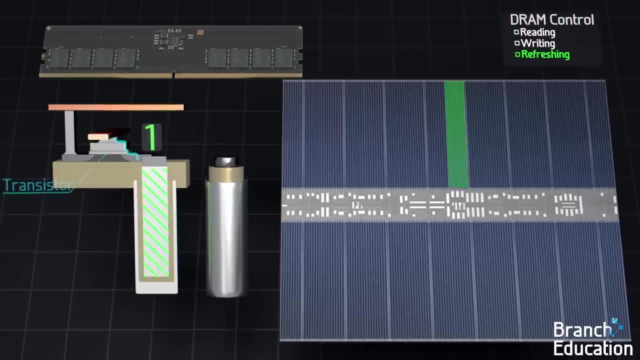 capacities, but is always in powers of 2.. Let's move on and discuss the third operation, which is refreshing the memory cells in a bank. As mentioned earlier, the transistors used to isolate the capacitors are incredibly small, and thus charges leak across the channel. 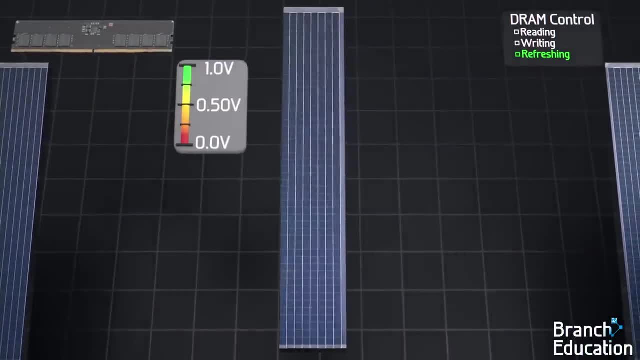 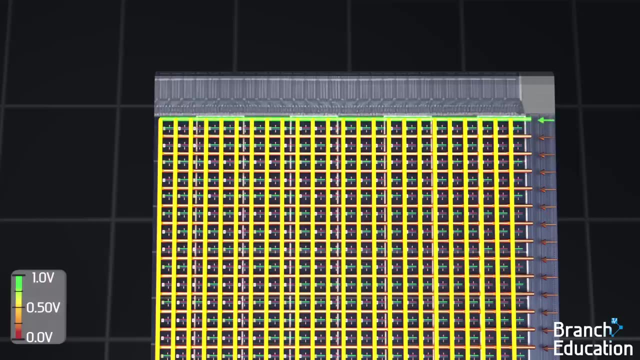 The refresh operation is rather simple and is a sequence of closing all the rows pre-charging, recharging the bit lines to 0.5 volts and opening a row To refresh just as before. the capacitors perturb the bit lines and then the sense amplifiers drive the bit lines and 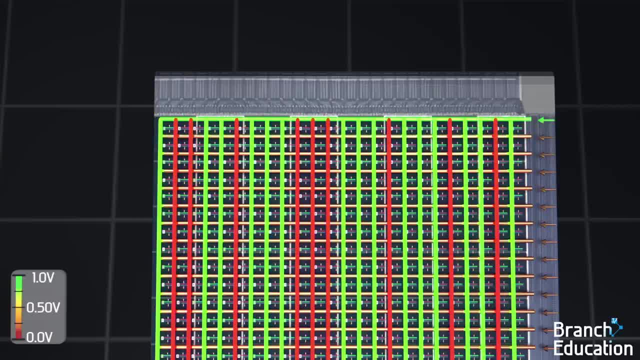 capacitors to the open row fully up to 1 volt or down to 0 volts, depending on the stored value of the capacitor, thereby refilling the leaked charge. This process of row closing, pre-charging, opening and sense amplifying happens row. after row. This is done by taking 50 nanoseconds for each row until all 65,000-ish rows are refreshed, taking a total of 3 milliseconds or so to complete. The refresh operation occurs once every 64 milliseconds for each bank, because that's statistically below the worst-case. 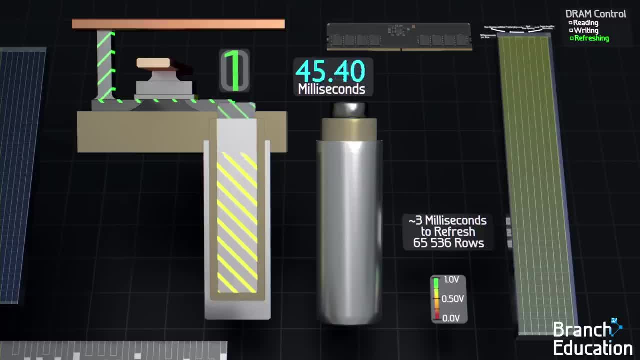 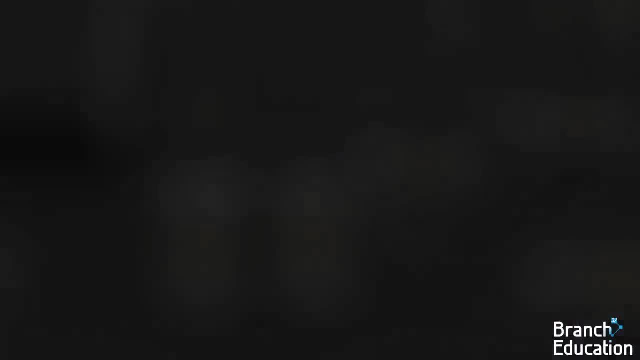 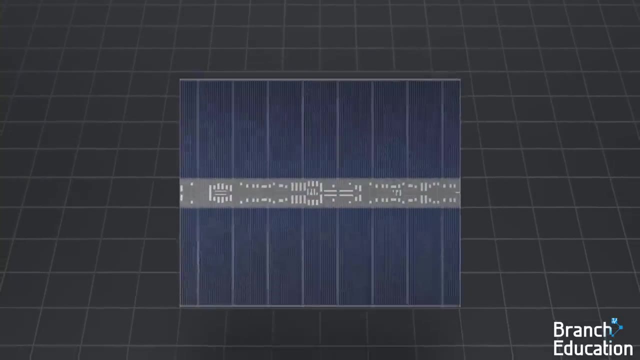 time it takes for a memory cell to leak too much charge to make a stored 1 turn into a 0, thus resulting in a loss of data. Let's take a step back And consider the incredible amount of data that is moved through DRAM memory cells. These 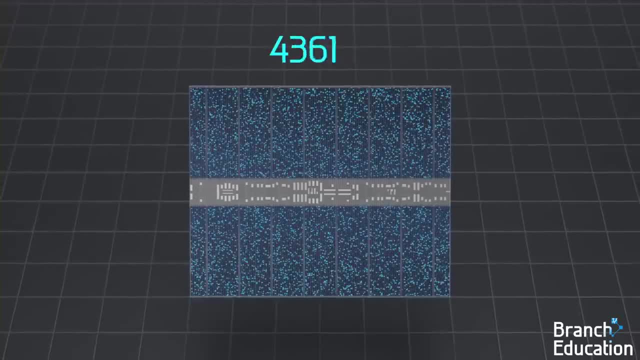 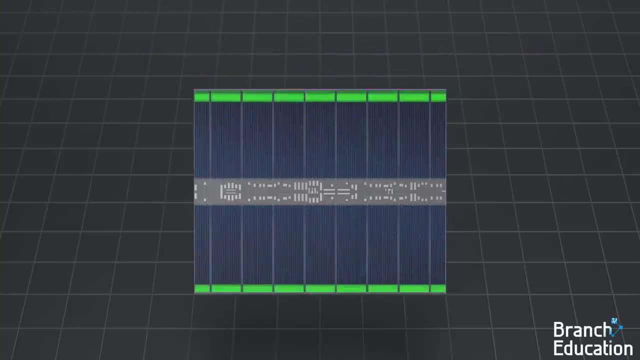 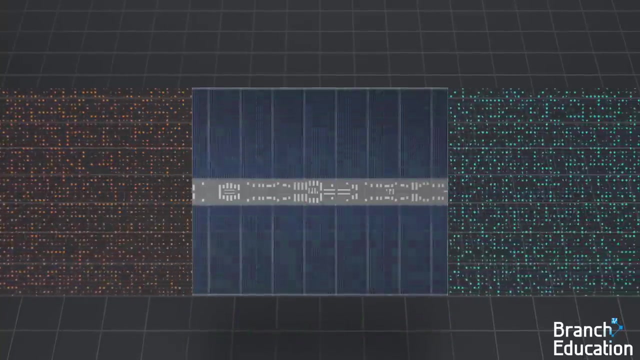 banks of memory cells handle up to 4,800 million requests to read and write data every second, while refreshing every memory cell in each bank, row by row, around 16 times a second. That's a staggering amount of data movement and illustrates the true strength of computers. 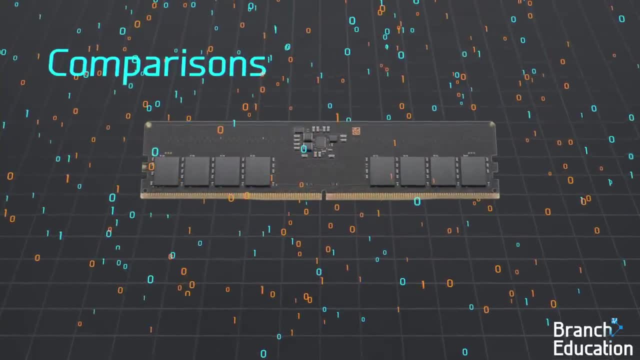 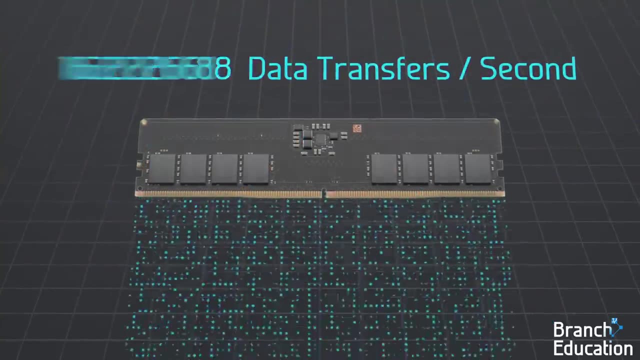 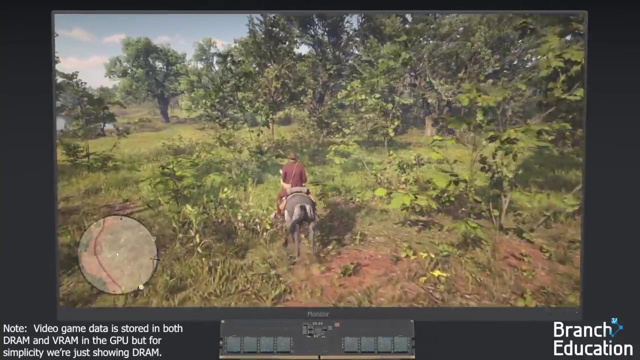 Yes, they do simple things like comparisons, arithmetic and moving data around, but at a rate of billions of times a second. Now you might wonder why computers need to do so much data movement. Well, take this video game, for example. You have obvious calculations, like the movement of your character. 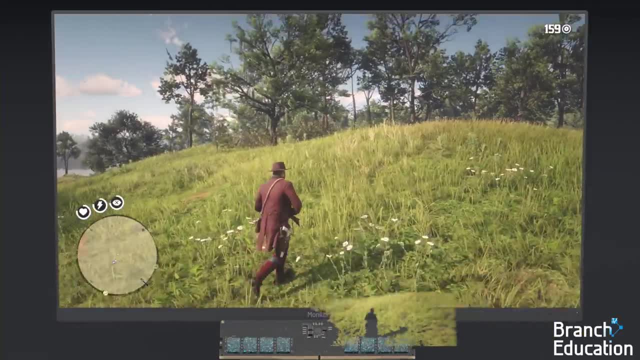 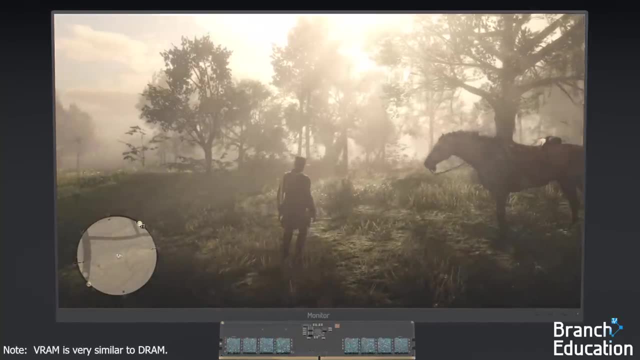 in a horse, But then there are individual grasses, trees, rocks and animals, whose positions and geometries are stored in DRAM, And then the environment, such as the lighting and shadows, change the colors and textures of the environment in order to 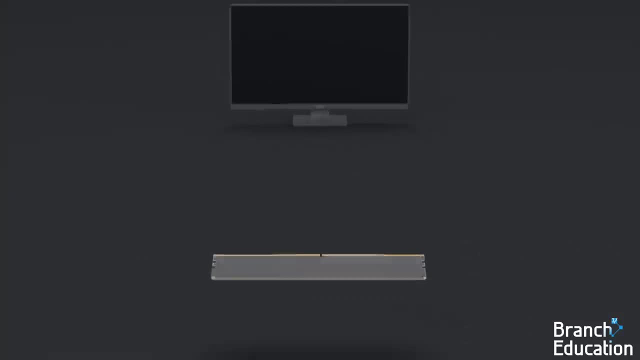 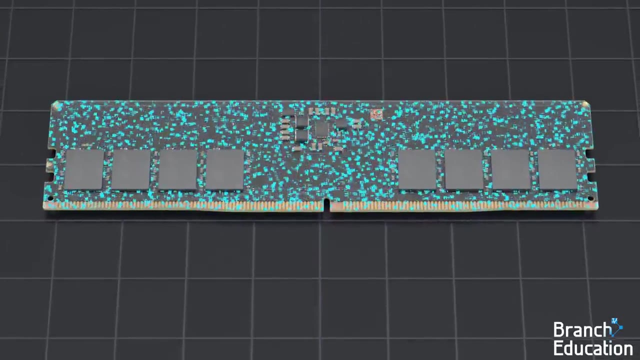 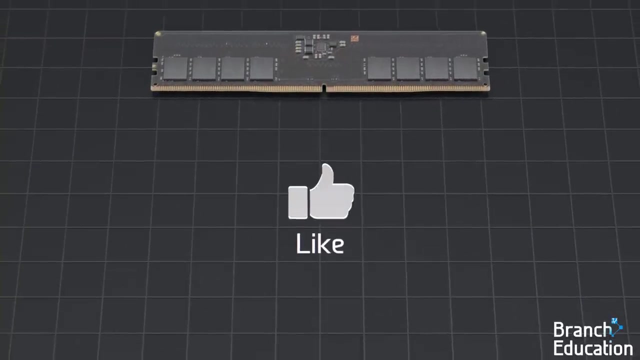 create a realistic world. Next we're going to explore breakthroughs and optimizations that allow DRAM to be incredibly fast. But before we get into all those details, we would greatly appreciate it if you could take a second to hit that like button, subscribe, if you haven't already, and type up a quick. 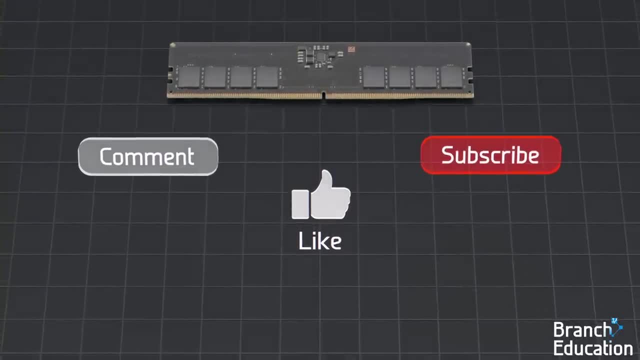 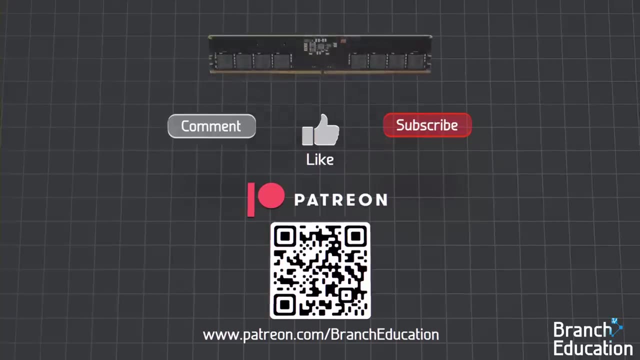 comment below, As it helps get this video out to our viewers. Thanks for watching. Also, we have a Patreon and would appreciate any support. This is our longest and most detailed video by far, and we're planning more videos that get into the inner details. 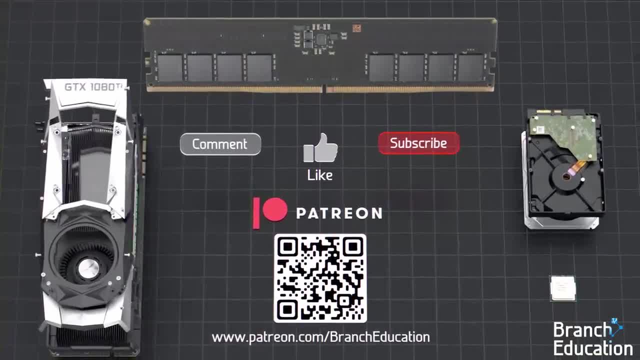 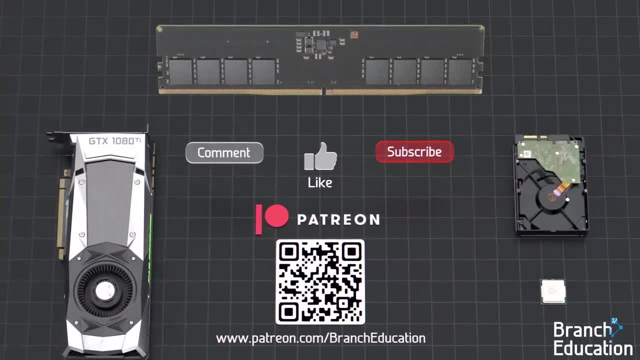 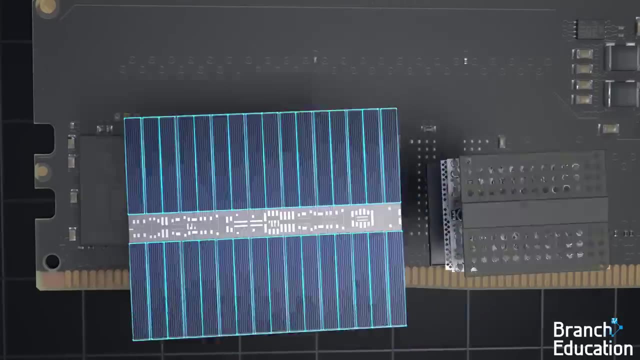 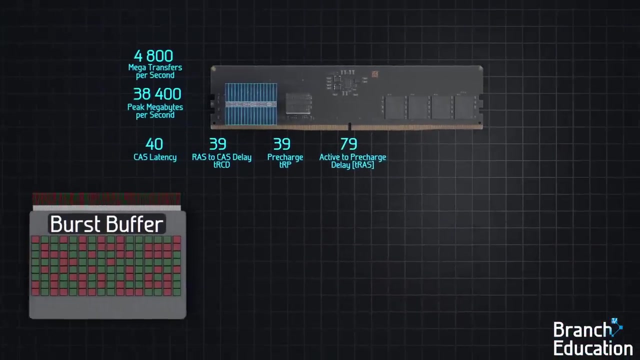 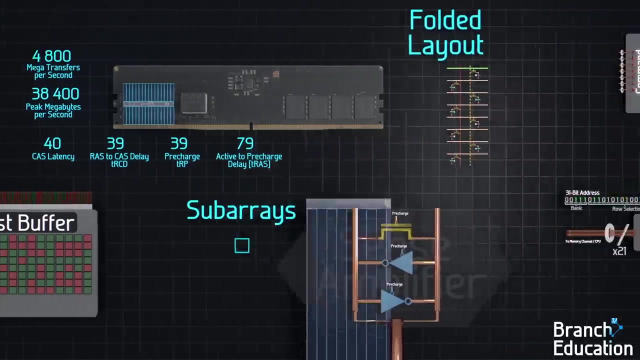 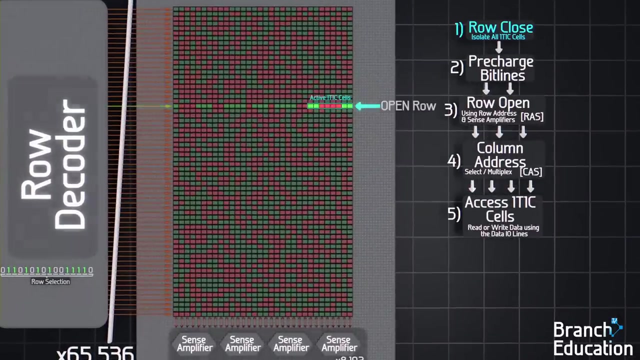 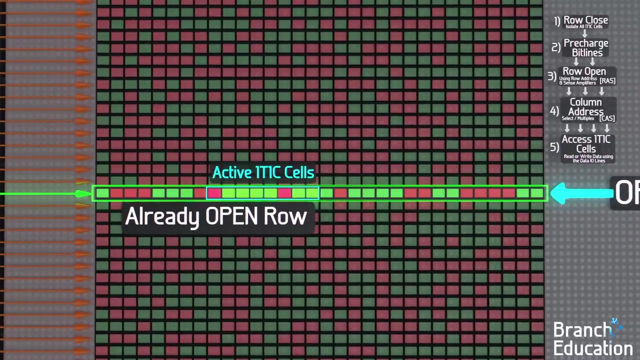 of how computers work. We can't do it without your help, So thank you for watching And doing these three quick things. It helps a ton. The first complex topic which we'll explore is why there are 32 banks. Let's look at a bank and what it's. 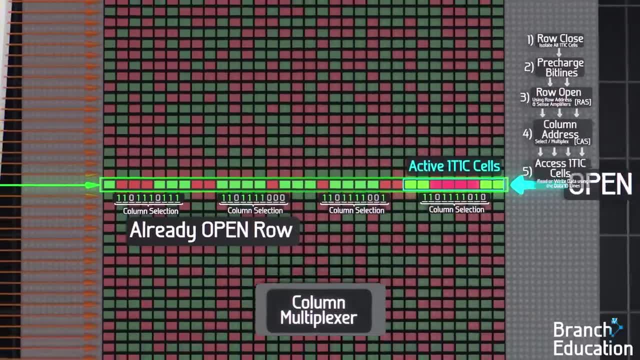 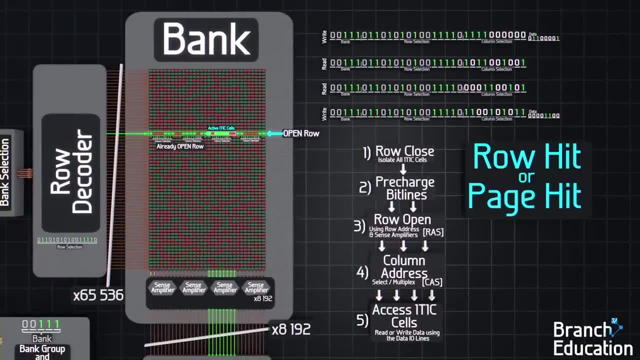 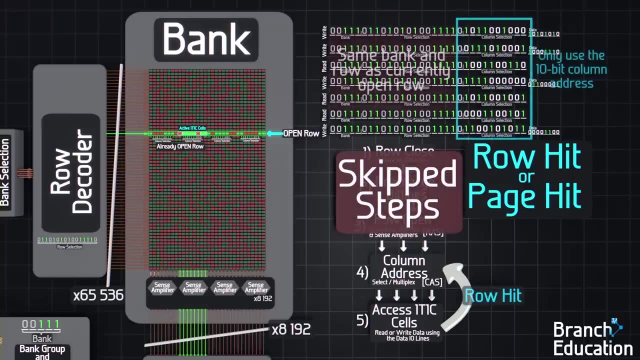 address and the column select multiplexer. When the CPU sends a read or write command to a row that's already opened, it's called a row hit or page hit, and this can happen over and over. With a row hit, we skip all the steps required to open a row and just use the 10-bit column address to 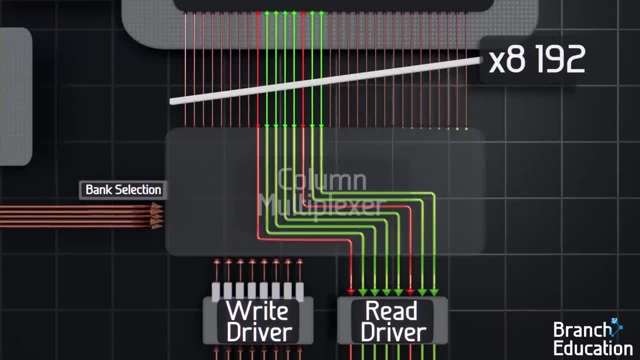 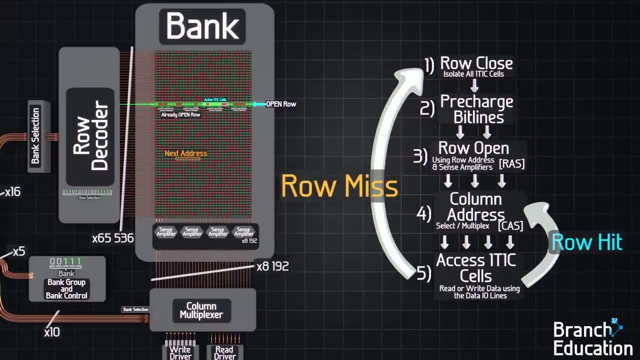 multiplex a different set of eight columns or bit lines, connecting them to the read or write driver, thereby saving a considerable amount of time. A row miss is when the next address is for a different row, which requires the DRAM to close and isolate the currently open row and then open. 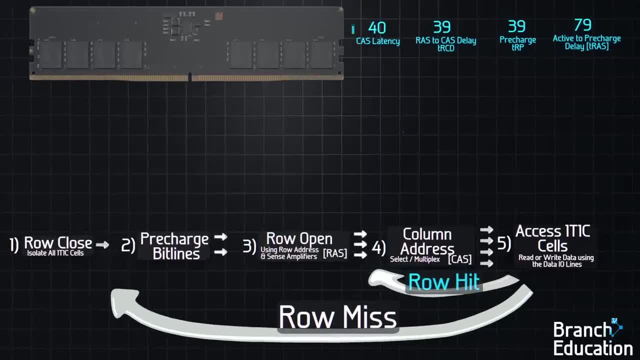 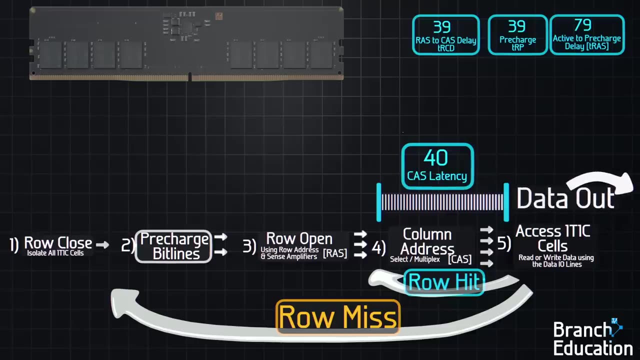 the new row. On a package of DRAM, there are typically four numbers specifying timing parameters regarding row hits, pre-charging and row misses. The first number refers to the time it takes between sending an address with a row open- thus a row hit- to receiving the data stored in the 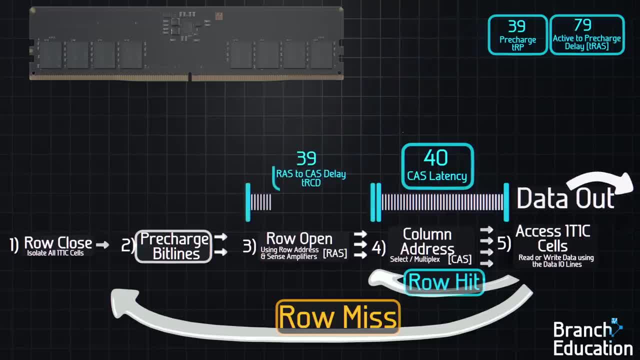 local address. This number is a complete link to the current address. for the first row, This is a columns. The next number is the time it takes to open a row. if all the lines are isolated and the bit lines are pre-charged, Then the next number is the. 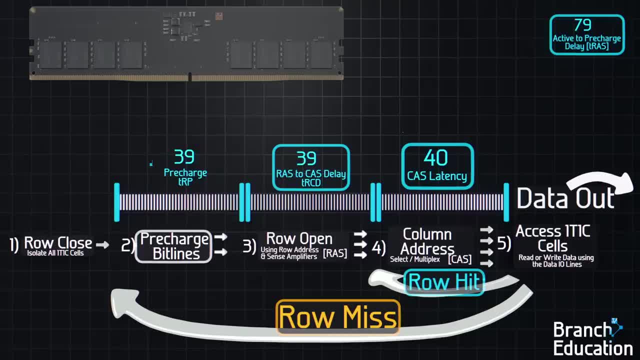 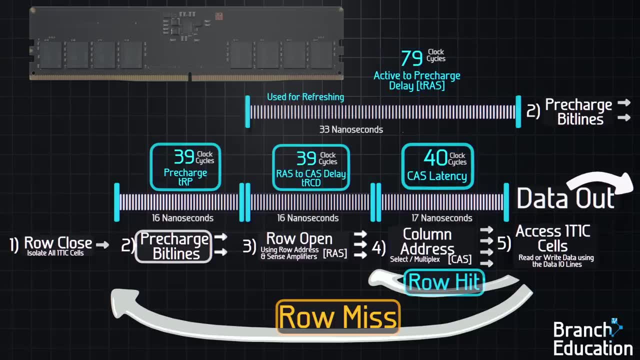 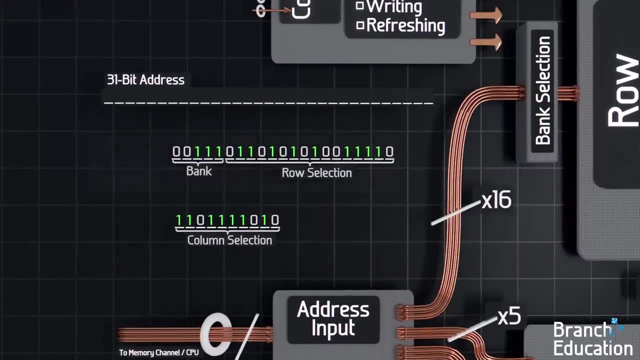 time it takes to pre-charge the bit lines before opening a row. And the last number is the time it takes between a row activation and the following pre-charge. Note that these numbers are measured in clock cycles. Row hits are also the reason why the address is sent in two sections. First, the bank selection. 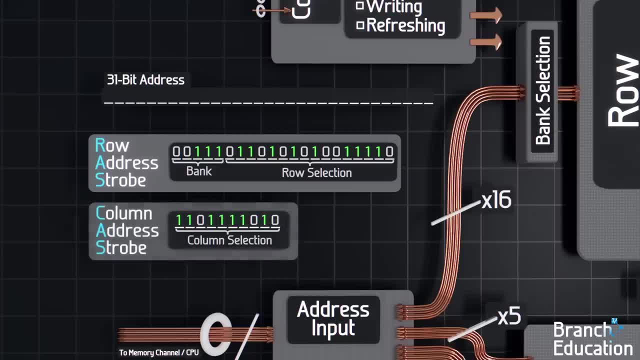 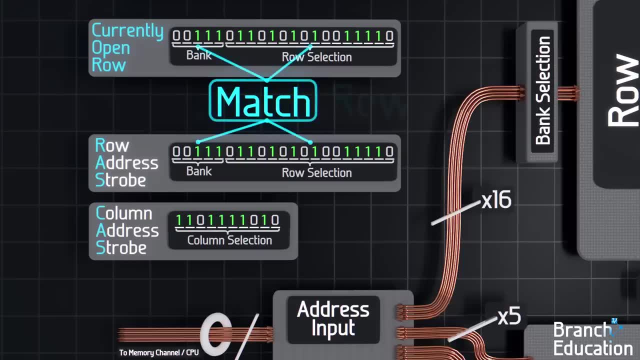 and row address called RAS and then the column address called CAS. If the first part, the bank selection and row address, matches a currently open row, then it's a row hit and all the DRAM needs is the column address and the new command. and 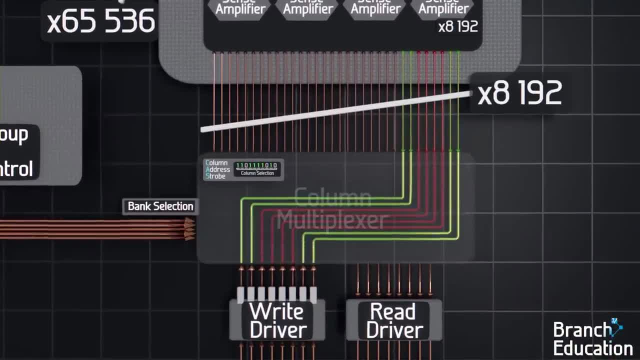 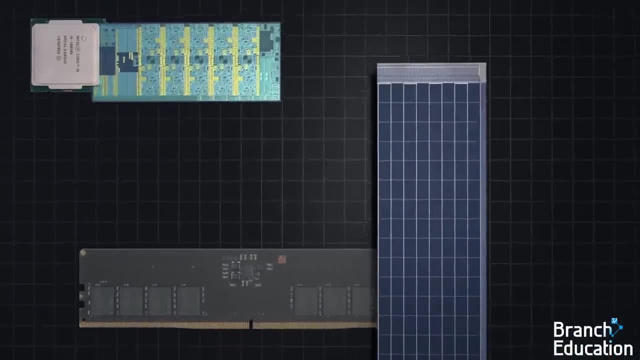 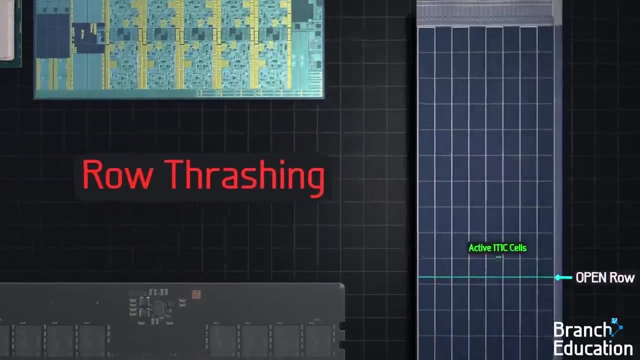 then the multiplexer simply moves around the open row. Because of the time saving and accessing an open row, the CPU memory controller programs and compilers are optimized for increasing the number of subsequent row hits. The opposite, called thrashing, is when a program jumps around from one row to a. 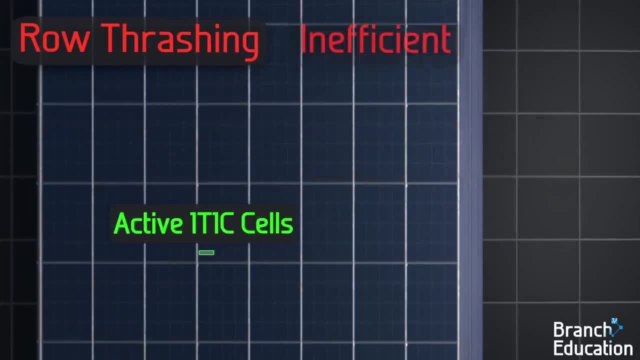 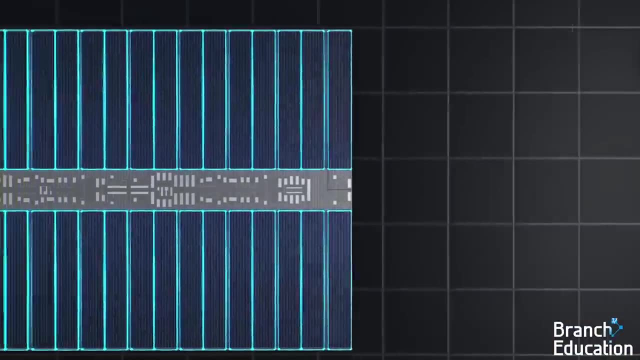 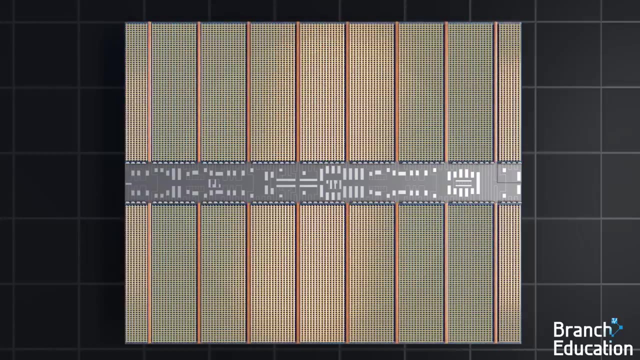 different row over and over and is obviously incredibly inefficient, both in terms of energy and time. Additionally, DDR5 DRAM has 32 banks. for this reason, Each bank's rows, columns, sense amplifiers and row decoders operate independently of one another and thus multiple rows from different banks can. 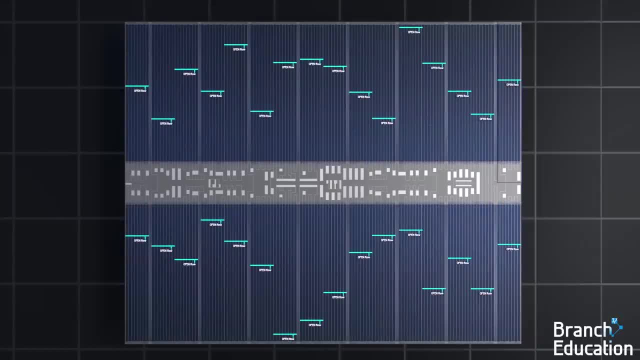 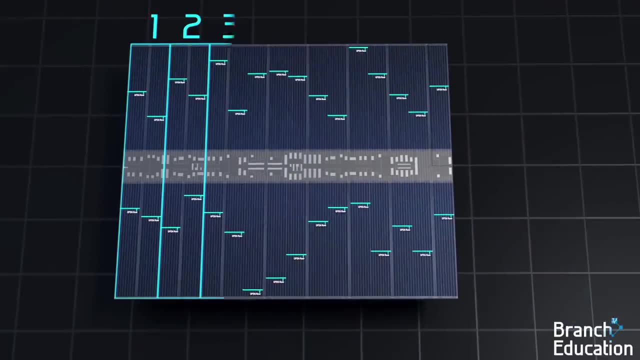 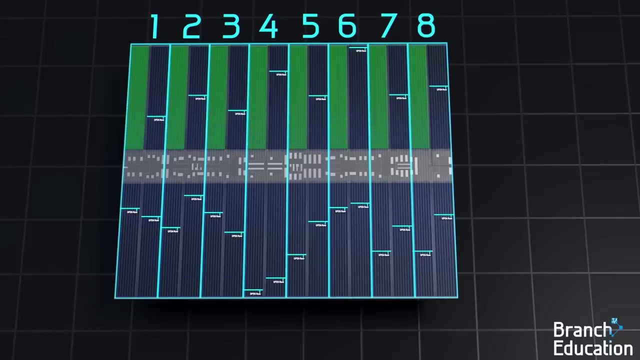 be open all at the same time, Increasing the likelihood of a row hit and reducing the average time it takes for the CPU to access data. Furthermore, by having multiple bank groups, the CPU can refresh one bank in each bank group at a time, while using the other three. 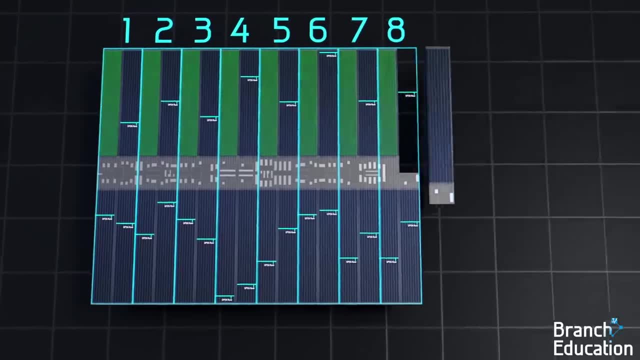 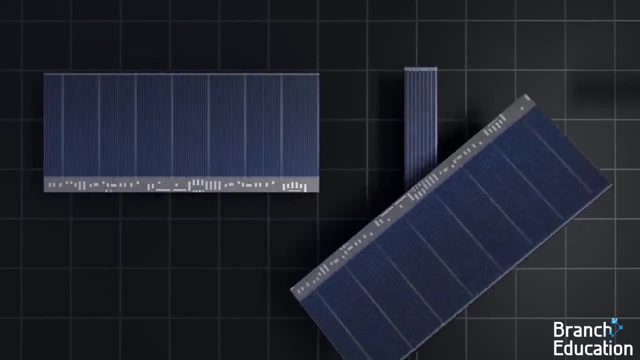 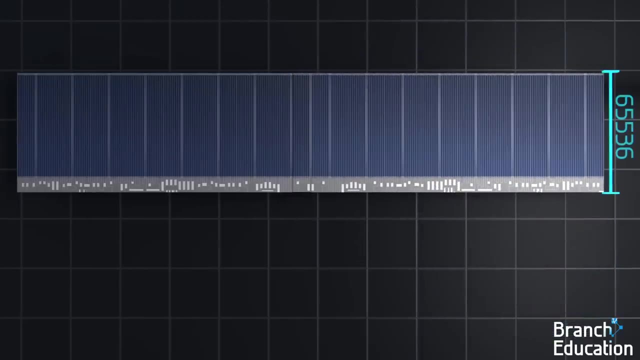 thus reducing the impact of refreshing. A question you may have had earlier is: why are banks significantly taller than they are wide? Well, by combining all the banks together, one next to the other, you can think of this chip as actually being 65,000 rows tall by 262,000 columns wide. And by adding 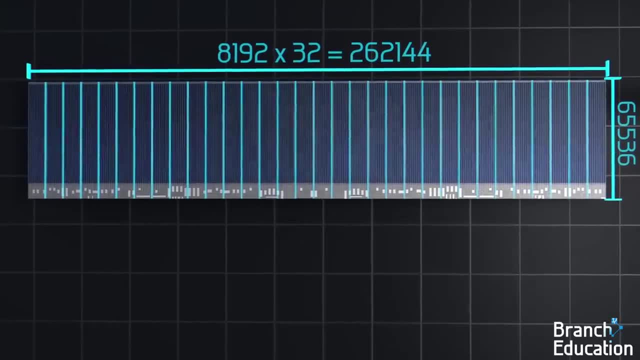 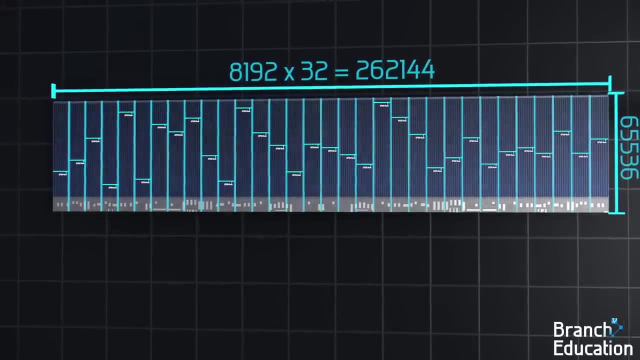 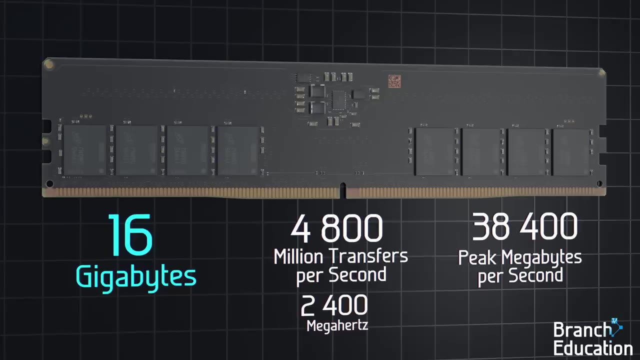 31 equally spaced divisions between the columns, thus creating banks. we allow for much more flexibility and efficiency in reading, writing and refreshing. Also note that on the DRAM packaging are its capacity in gigabytes, the number of millions of data transfers per second and the number of data transfers per second. 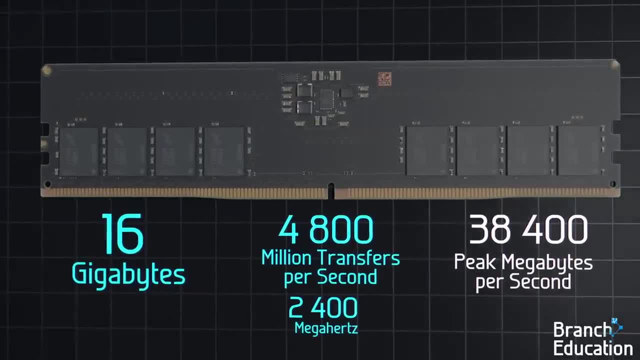 Also note that on the DRAM packaging are its capacity in gigabytes, the number of millions of data transfers per second and the number of data transfers per second. The ratio of data concentration to rebounds is 2 times the clock frequency and the peak. 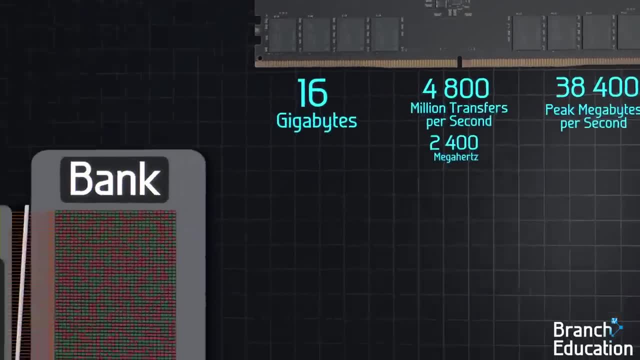 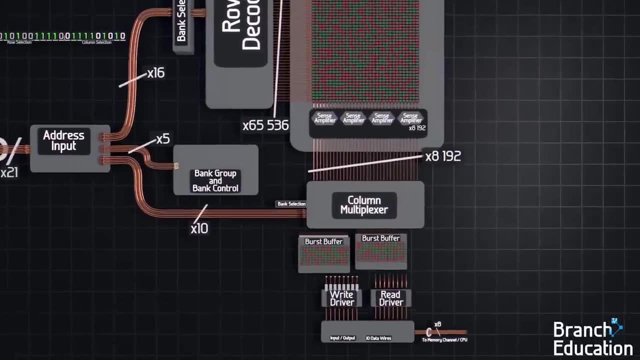 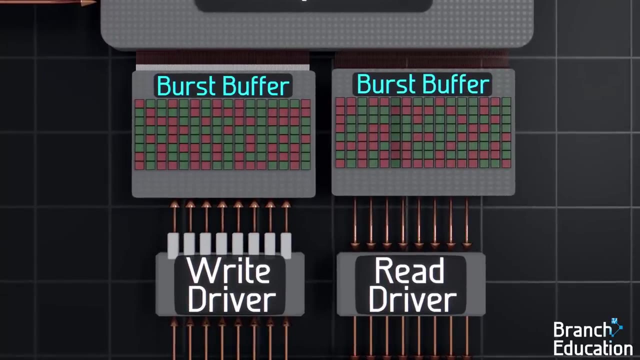 data transfer rate in megabytes per second. The next design optimization we'll explore is the burst buffer and burst length. Let's add a 128-bit read and write temporary storage location, called a burst buffer, to our Functional Diagram, Instead of 8 wires coming out of the multiplexer. 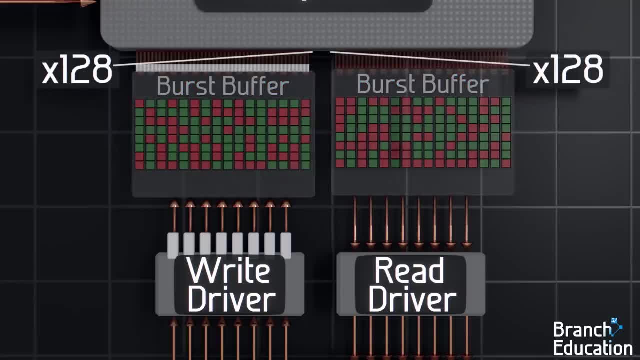 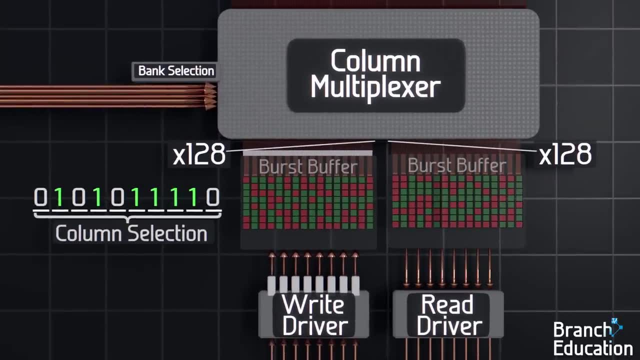 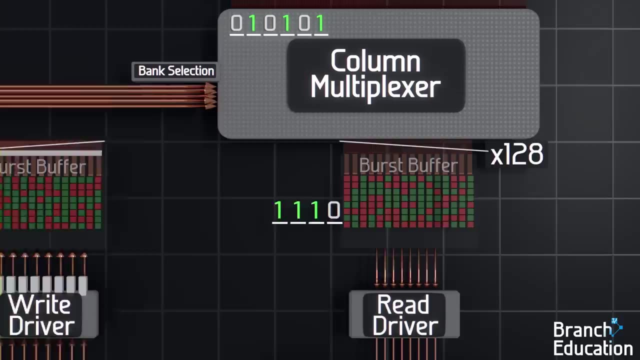 we're going to have 128 wires that connect to these 128 bit buffer locations. Next, the 10-bit column address is broken into two parts. Six bits are used for the multiplexer and four bits are for the burst buffer. Let's explore a reading command. 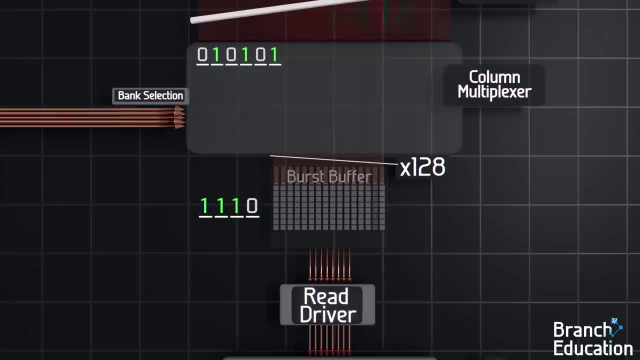 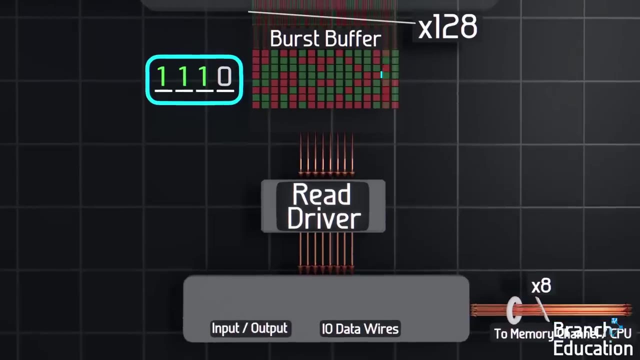 With our burst buffer in place, 128 memory cells and bitlines are connected to the burst buffer using the six column bits, thereby temporarily loading or caching 128 values into the burst buffer. Within the four bits for the buffer, eight quickly accessed data locations in the burst. 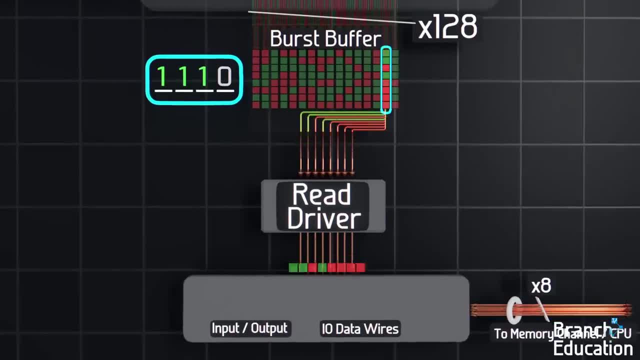 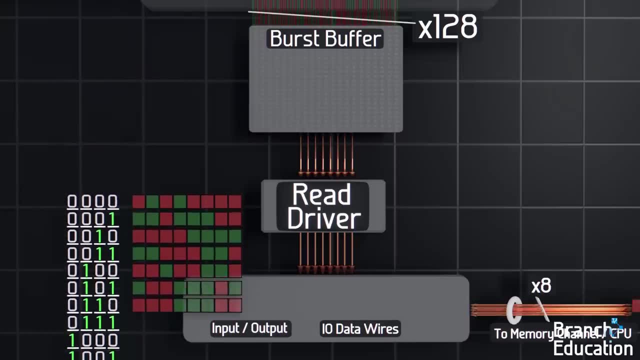 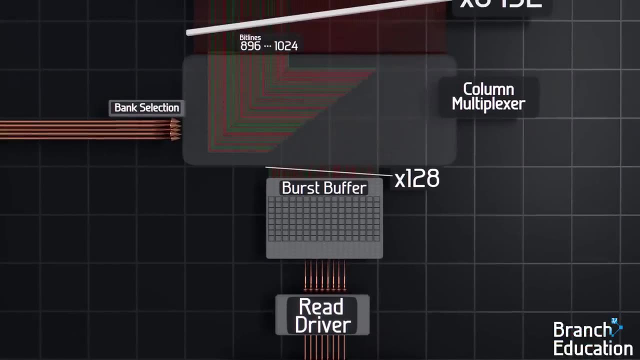 buffer are connected to the read drivers and the data is sent to the CPU. By cycling through these four bits, all 16 sets of eight bits are read out, and thus the burst length is 16.. After that, a new set of 128 bitlines and values are connected and loaded into the burst. 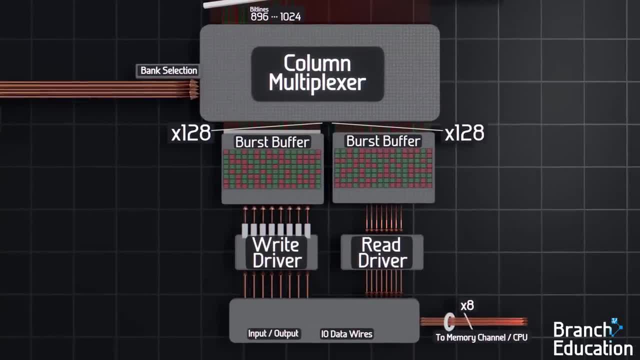 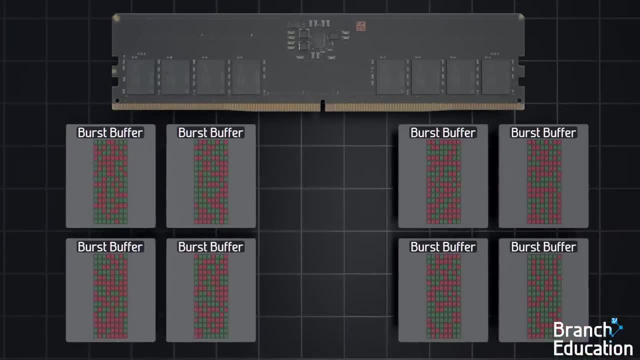 buffer. There is also a write burst buffer which operates in a similar way. The benefit of this system is that the data is sent to the CPU. The next design is that 16 sets of 8 bits per microchip, totaling 1,024 bits, can be accessed. 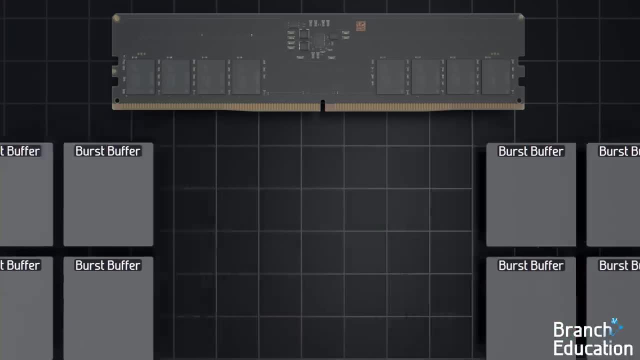 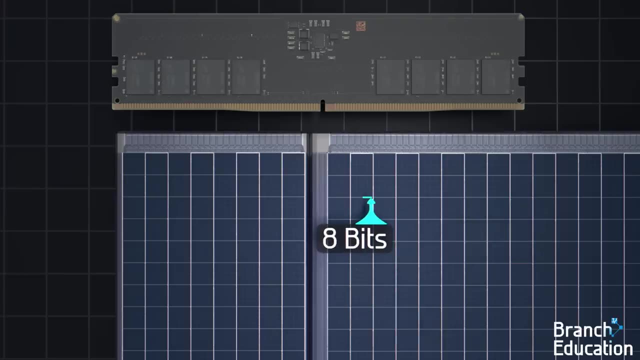 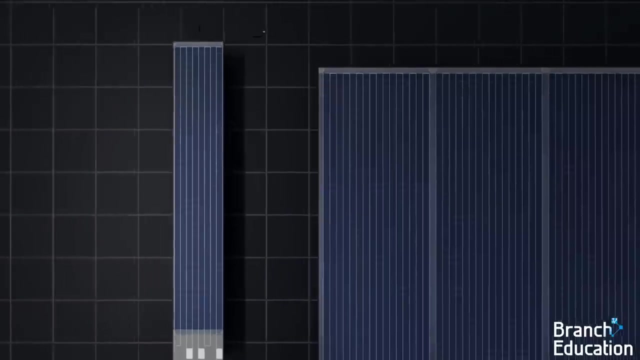 and read or written extremely quickly, as long as the data is all next to one another, But at the same time we still have the granularity and ability to access any set of 8 bits if our data requests jump around. The next design optimization is that this bank of 65,536 rows by 8,100 bits can be. 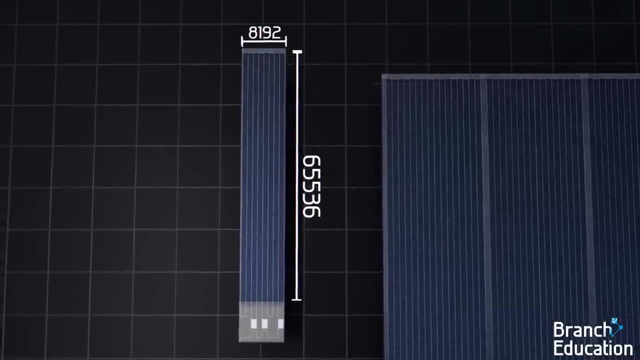 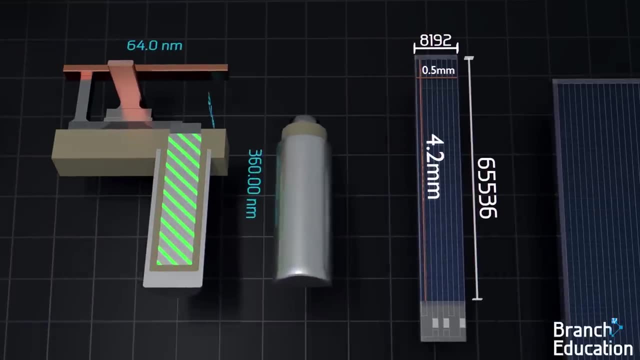 loaded into the burst buffer. The result of thisützenation is that the maximum number of words that are in these 192 columns are relatively massive and are extremely long word lines and bitlines, especially when compared to the size of each trench capacitor memory cell. 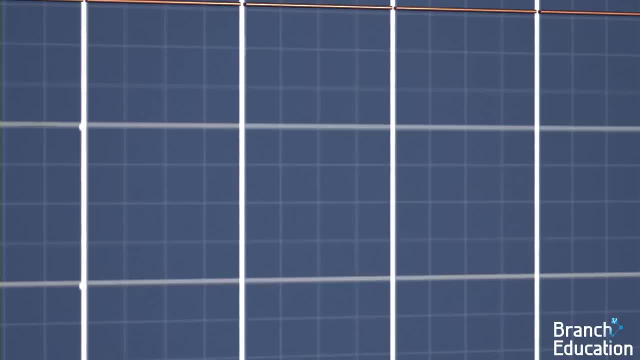 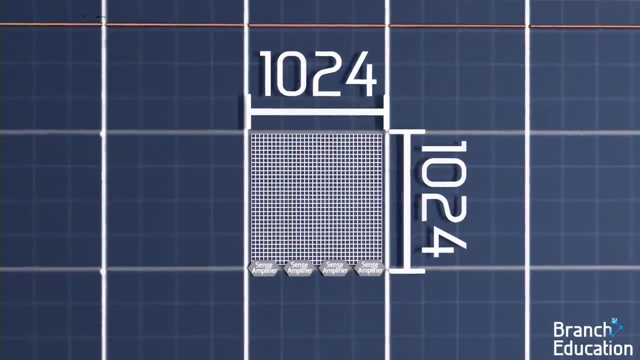 Therefore, the massive array is broken up into smaller blocks, 1024 by 1024, with intermediate sense amplifiers below each subarray and subdividing wordlines, and using a hierarchical row decoding scheme. By subdividing the bitlines, each wordline is divided into two parts, which means that each of these parts supersedes each other by a zero. Where there's a small increase in each wordline, 1,024 is put in a smaller block and the rest- Every other wordline- is put in a small block. the distance and amount of wire that each tiny capacitor is connected to as it perturbs the bit line to the sense amplifier is reduced, and thus the capacitor doesn't have to be as big. By subdividing the word lines, the capacitive load from 8,000-ish transistor gates and channels is decreased. 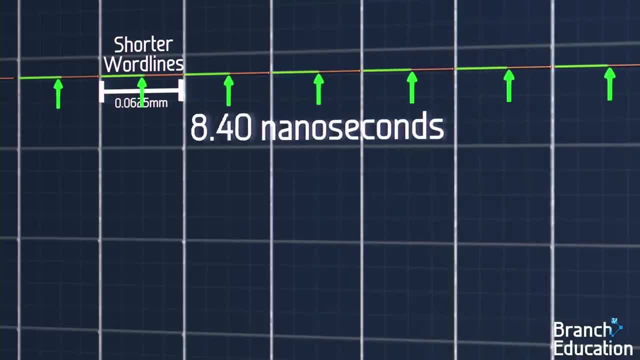 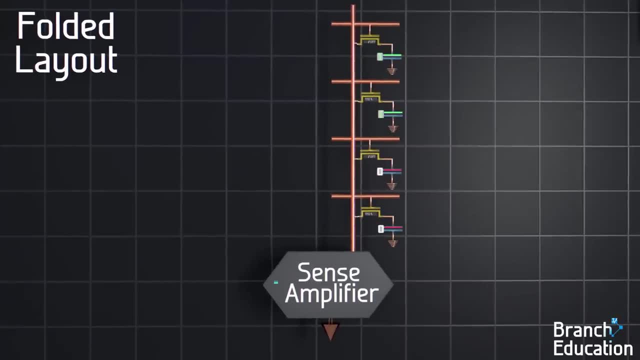 and thus the time it takes to turn on all the access transistors in a row is decreased. The final topic we're going to talk about is the most complicated. Remember how we had a sense amplifier connected to the bottom of each bit line. 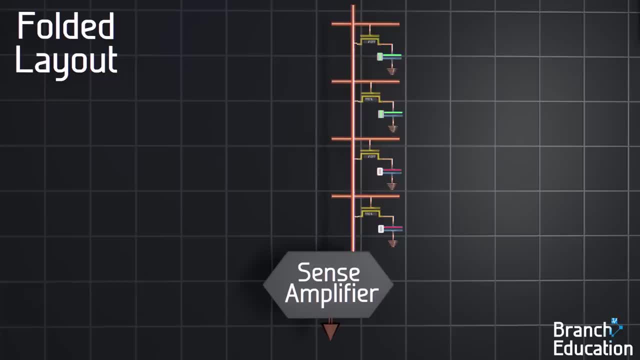 Well, this optimization has two bit lines per column going to each sense amplifier and alternating rows of memory cells connected to the left and right bit lines, thus doubling the number of bit lines. When one row is active, half of the bit lines are active. 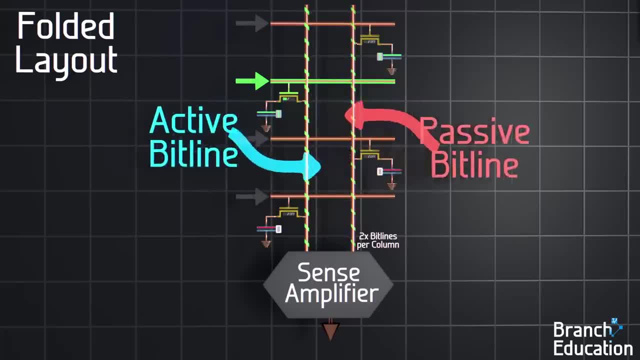 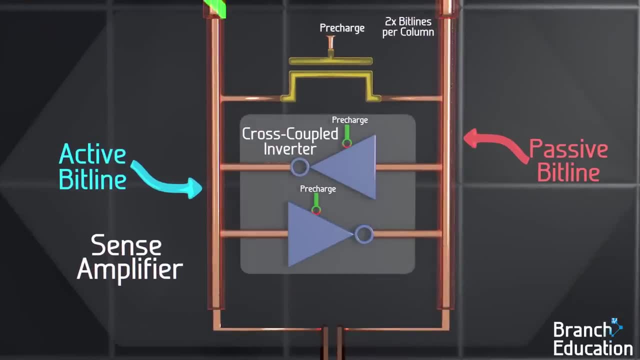 while the other half are passive, and vice versa when the next row is active. Moving down to see inside the sense amplifier, we find a cross-coupled circuit. How does this work? Well, when the active bit line is a 1,. 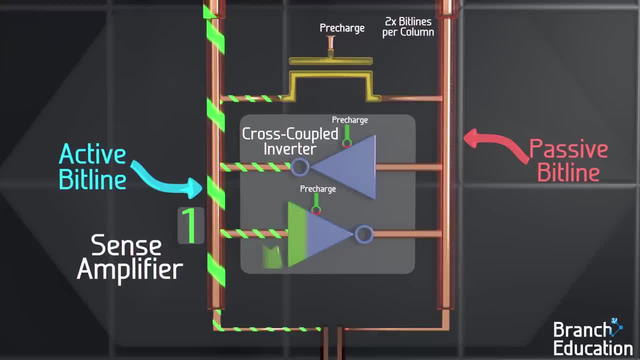 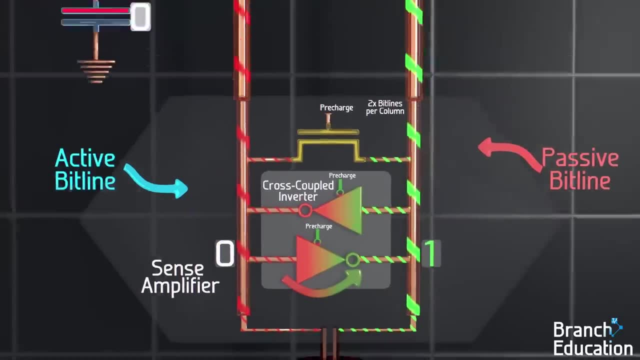 the passive bit line will be driven by this cross-coupled inverter to the opposite value of 0, and when the active is a 0,, the passive becomes a 1.. Note that the inverted passive bit line isn't connected to any memory cells. 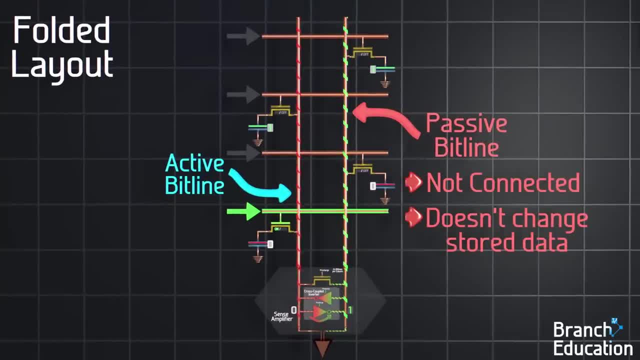 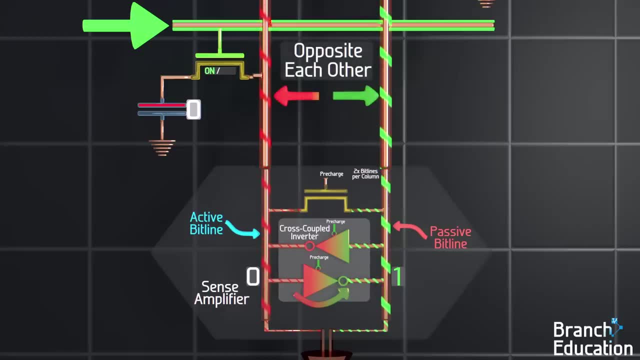 and thus it doesn't mess up any stored data. The cross-coupled inverter makes it such that these two bit lines are always going to be opposite one another, and they're called a differential circuit. Now what does that mean? Well, it's a differential pair. 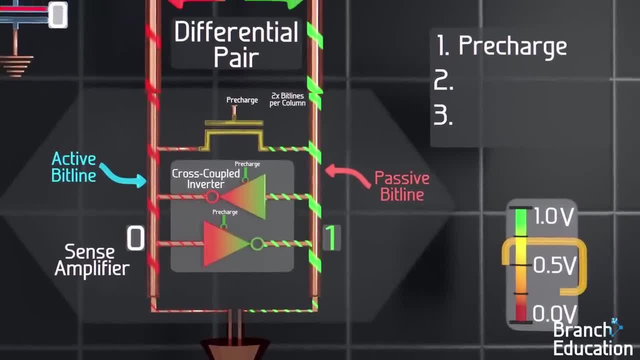 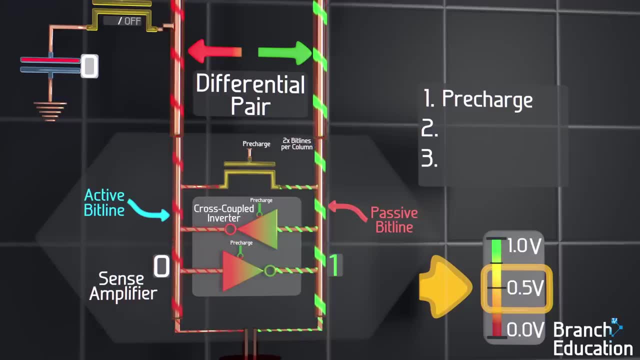 There are three benefits to this design. First, during the pre-charge step, we want to bring all the bit lines to 0.5 volts and, by having a differential pair of active and passive bit lines, the easiest solution is to disconnect the cross-coupled inverters. 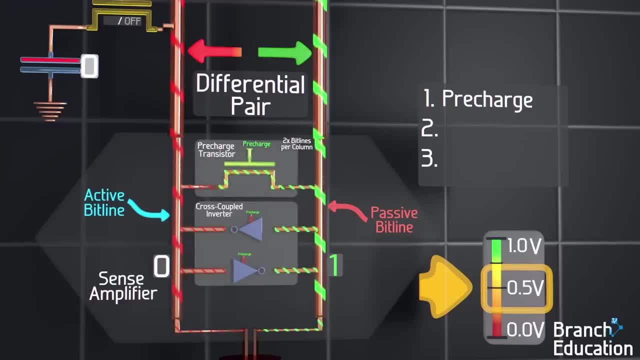 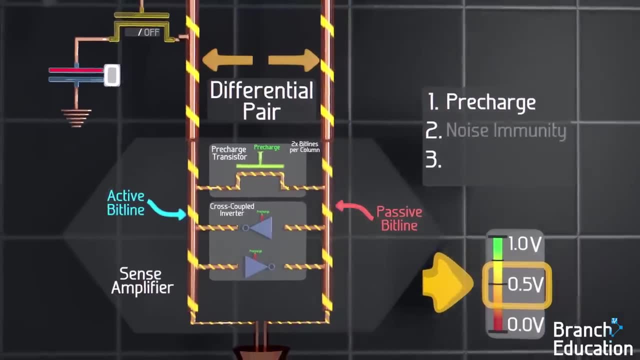 and open a channel between the two using a transistor. The charge easily flows from the 1 bit line to the 0, and they both average out and settle at 0.5 volts. noise immunity and a reduction in parasitic capacitance of the bit line: These benefits. 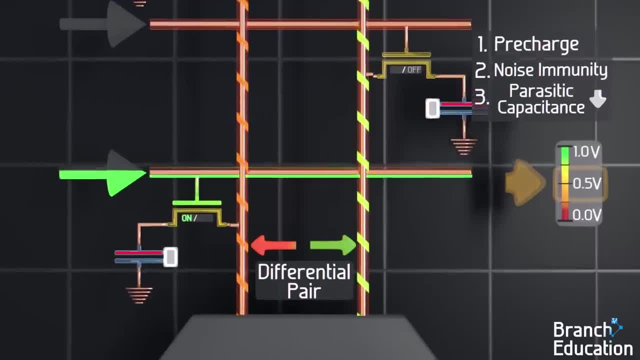 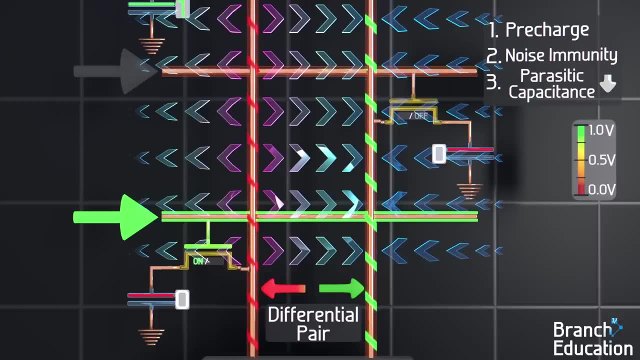 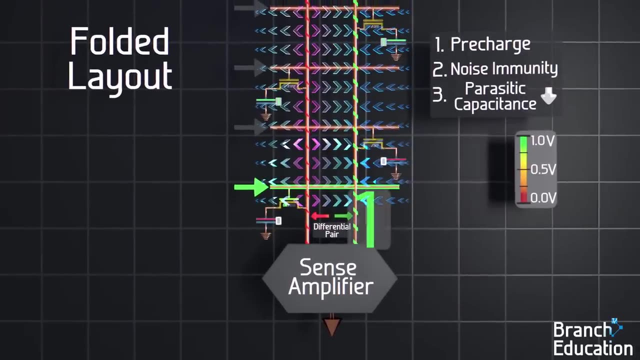 are related to the fact that, by creating two oppositely charged electric wires with electric fields going from one to the other, we reduce the amount of electric fields emitted in stray directions and, relatedly, increase the ability of the sense amplifier to amplify one bit line to one. 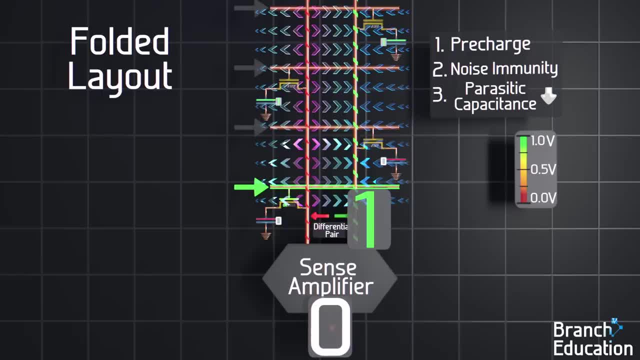 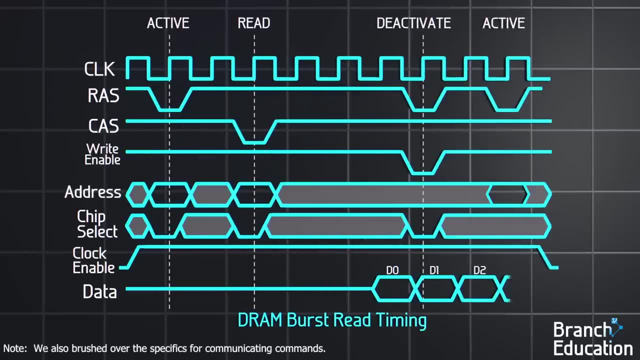 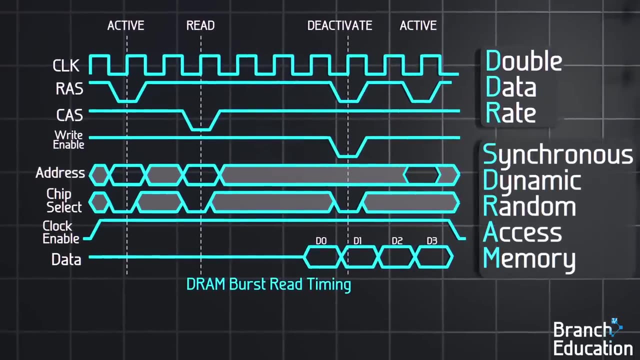 volt and the other to zero volts. One final note is that when discussing DRAM, one major topic is the timing of addresses, command signals and data and the related acronyms DDR, or double data rate, and SDRAM, or synchronous DRAM. These topics were omitted from this video because it would